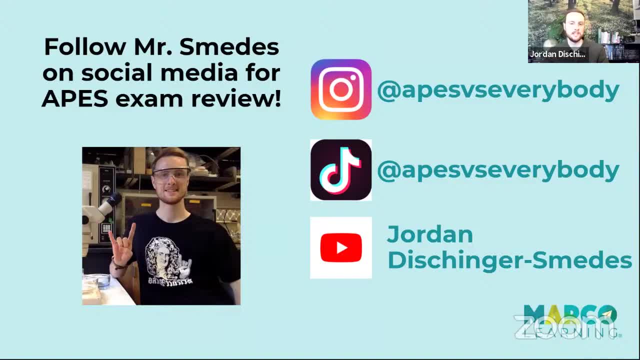 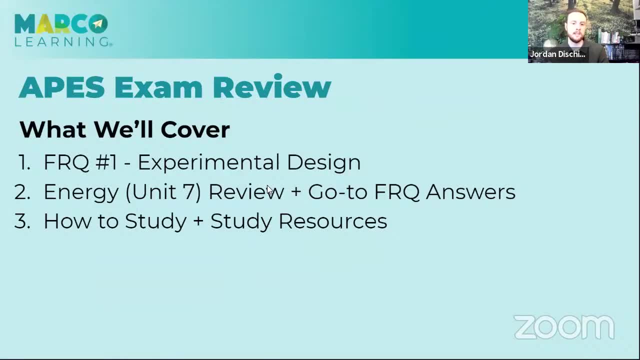 it and again, check me out on the socials, on TikTok. Just getting started, so not a lot of stuff there, but there's going to be more as the exam gets closer and closer. But what are we covering today? We're going to cover FRQ number one, which is the Experimental Design FRQ. We'll 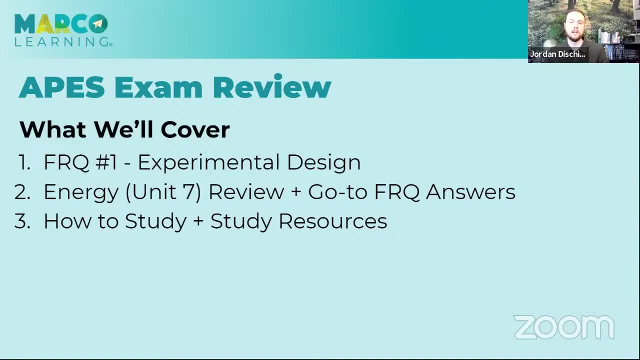 go through that a little bit later. So let's get started. So let's go through how you can make sure to earn as many points as possible on this- tips and tricks, things to avoid and things to make sure you do. Then we'll do some content. 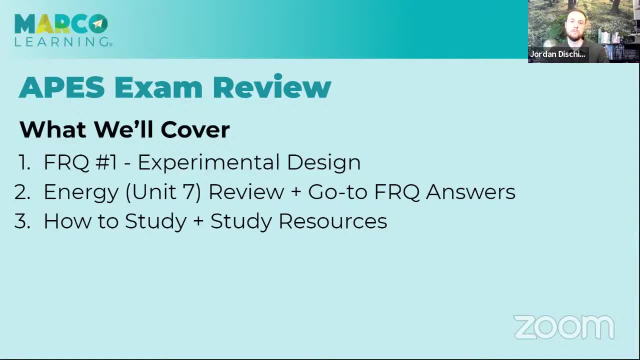 review unit seven, which is going to cover atmospheric pollution, or what you might call air pollution, And we're going to review go-to FRQ answers- things you need to understand- for unit seven, And then we'll wrap up with a really quick: how should you study and what resources? 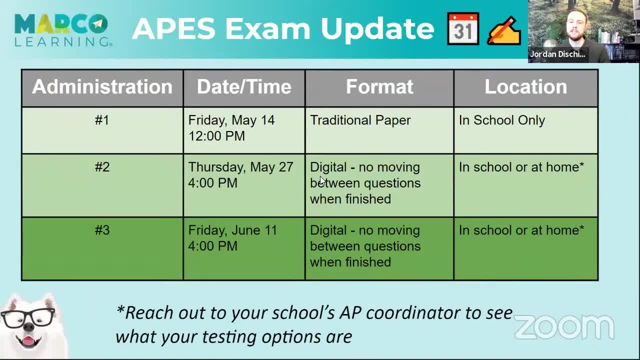 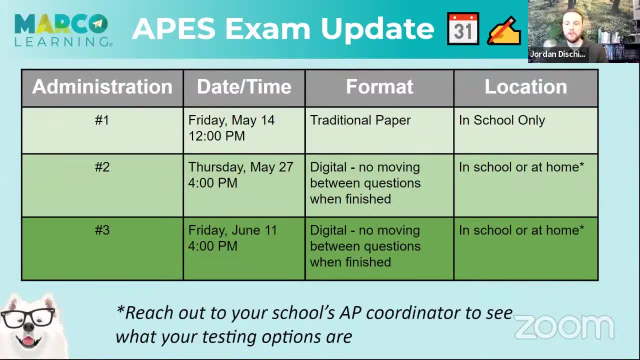 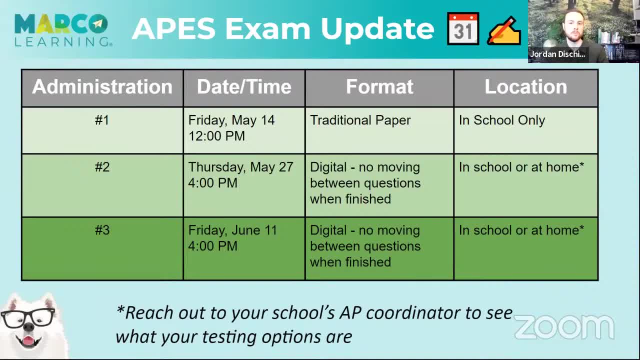 That might be because you're taking the June 11th exam And so you have to talk with your teacher and with your school to figure out when your exam date is. Now I'll be doing a lot of YouTube content. John and I will be doing a last minute age review on the 12th or the 13th, maybe both. 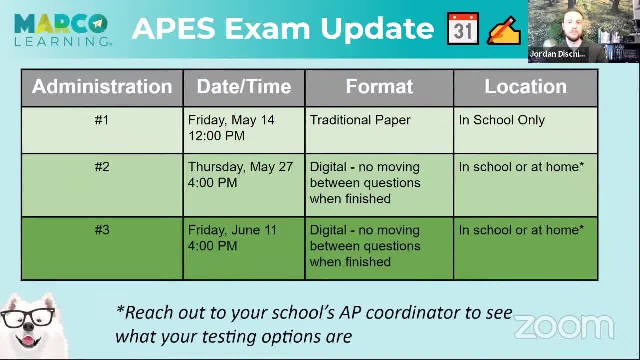 right before that 14th exam, which a lot of you are taking, but I'll also be doing last minute review for the 27th and I'll be doing last minute review for the 11th, So no matter what exam you're. 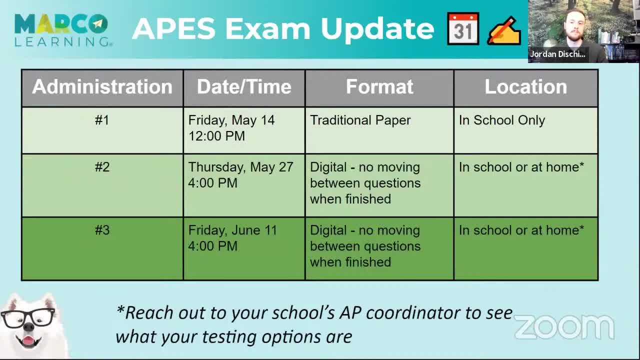 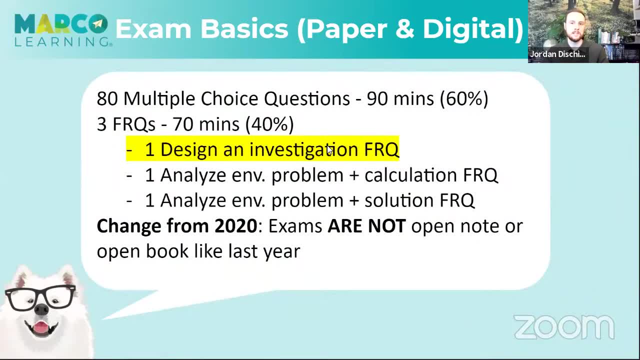 taking. I will be there for you. So I'll be doing a last minute review for the 11th. So, no matter what, walking you through the final couple of days of review for each of these exams, trying to make sure you go in as comfortable as possible. So what are the exam basics? 80 multiple choice questions. 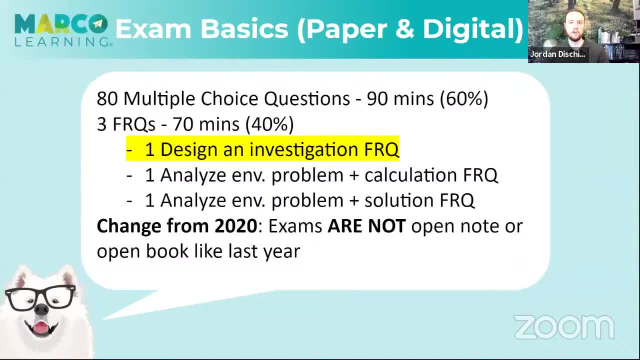 in 90 minutes. that's going to be 60% of your overall score. Then there are three FRQs. You'll have 70 minutes to write them and that's 40% of your overall score. That is going to break down. 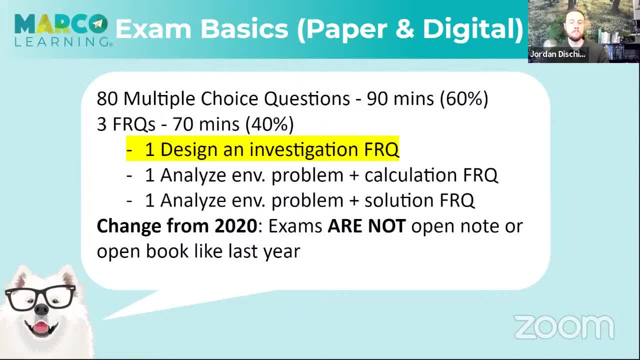 to about 23 minutes for a few, And I have coming out on my channel in the next couple of days the first video which we'll go through in depth: how to design an investigation, FRQ. We're going to touch on it in this video. 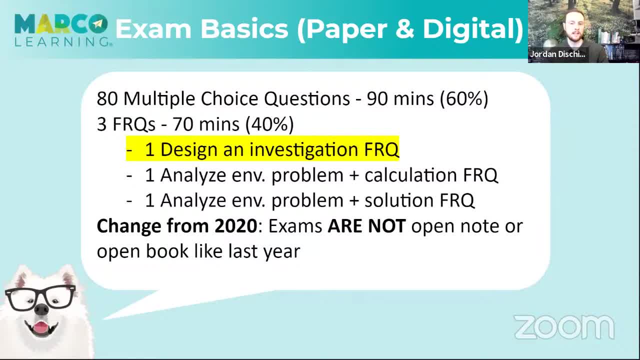 but I'm going to do a deep form analysis of that FRQ, go through exactly how to get ready for it. So you want to make sure you subscribe to my channel- if you don't already- and check that out there. Then we have the analyze, environmental problem and calculation FRQ. There'll be a video. 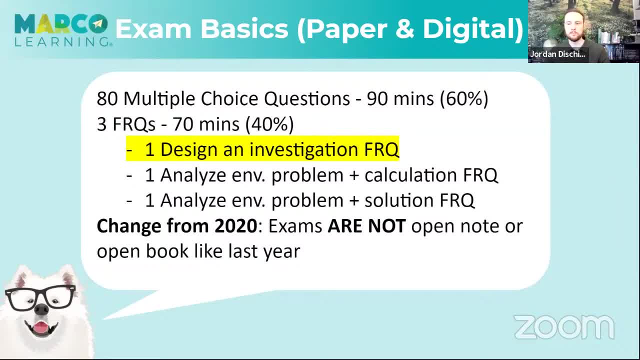 on my channel about that soon, as well as an environmental problem and proposing a solution. One thing to make sure you know is that the 2020 exam was open book open note, because you're at home. That is not the case in 2020.. So I'm going to go through in depth how to design an investigation. 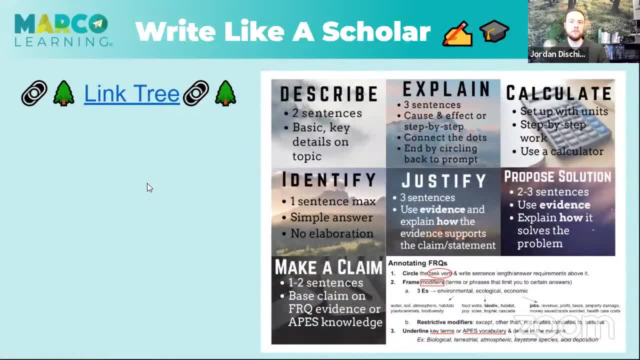 FRQ 2021.. So a new exam format. If you don't already have this link tree again, make sure to check this out. It'll be in the comments for this video. You want to make sure you have this FRQ. 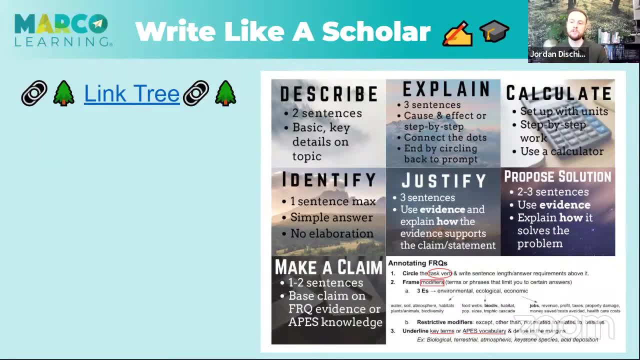 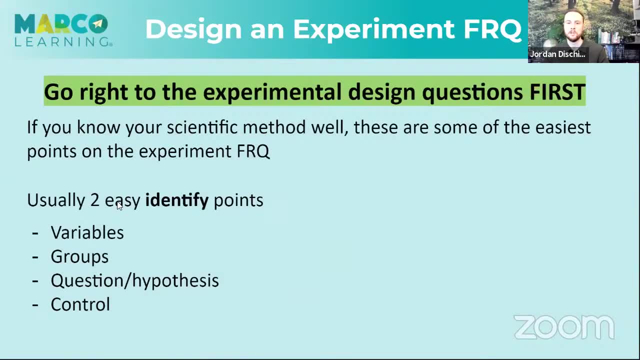 task verb sheet because I'll be referencing in this video and in future videos- identify, describe, explain, justify- Really helpful if you already know how to do that. So when we get to designing an FRQ, we need to understand that we want to go right to the design and FRQ portion. 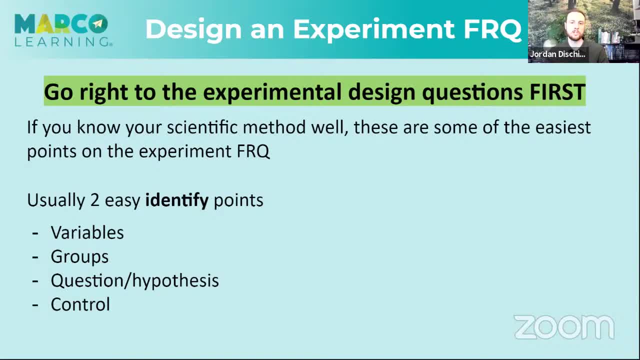 of this FRQ. So we want to skip to the questions that are about designing an experiment. They may not be the first question, but in my opinion they're some of the easiest, And so it makes sense to do them first so that you don't run out of time. So one thing I like to tell students is: 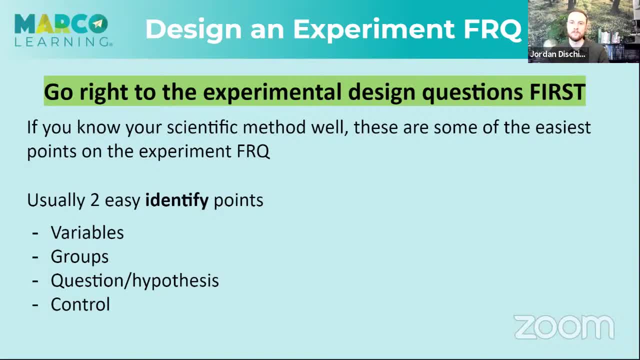 not all FRQ points are equal. They're all worth one point every question, in most cases sometimes two, but they are not all equally difficult to earn, And so we want to go right for those identified points. Now, when we're talking about an experiment, 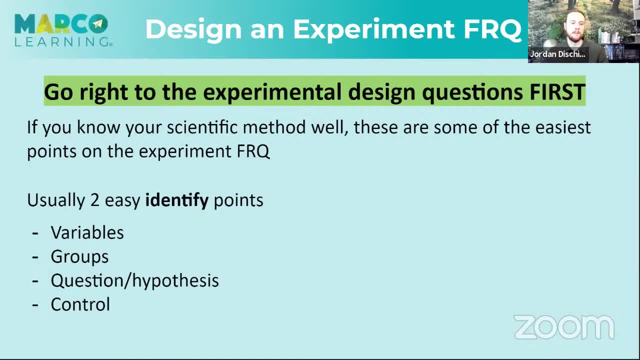 what are the things you might have to identify? Well, you might have to identify variables, You might have to identify groups, You might have to identify questions and that hypothesis and you might have to identify controls. And so let's go into how to do those things First. 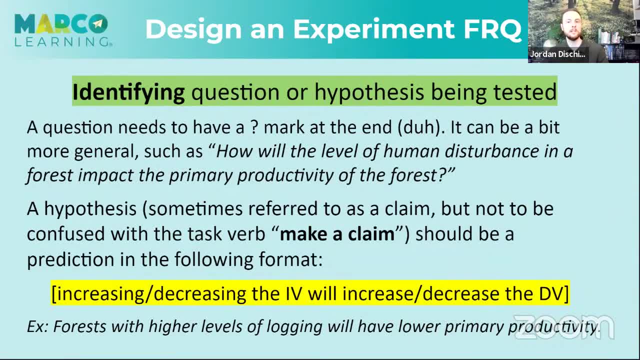 if you're identifying a question or hypothesis being tested, you need to be really clear that if it's a question, you have a question mark at the end. that might seem kind of obvious, but it's not obvious to everybody. Sometimes people want to write a hypothesis when they're 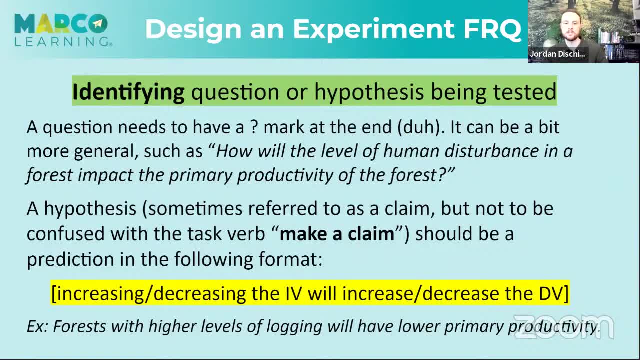 asked to write a question. So an example here would be: how will the level of human disturbance in a forest impact the primary productivity of the forest? That would be point worthy in terms of a question. We have a question mark. at the end We have: how will something impact something else? We'd be good to go If. 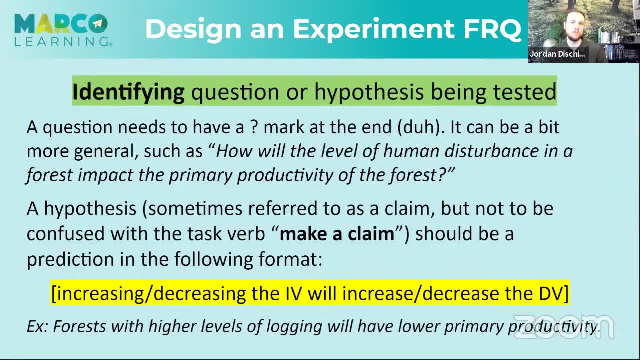 we're asked to identify a hypothesis, which will sometimes be referred to as a claim. but that's different than make a claim. If you're asked to make a claim, then you should justify and support it, But if you're just asked to identify a hypothesis or a claim of the investigator or 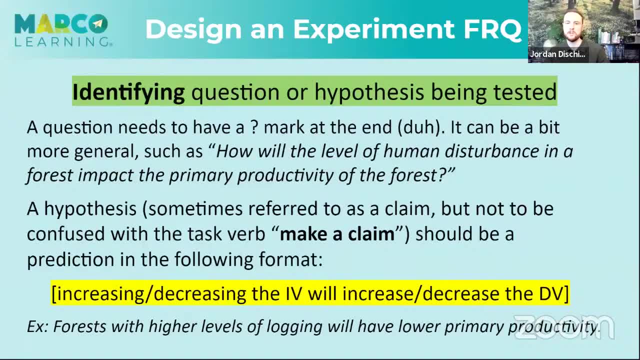 the scientist, then you're just going to have to make a claim. So if you're asked to identify a hypothesis, you're giving a one sentence answer. Now I have highlighted in yellow here a very simple template that you want to use anytime you identify a hypothesis Increasing or decreasing the 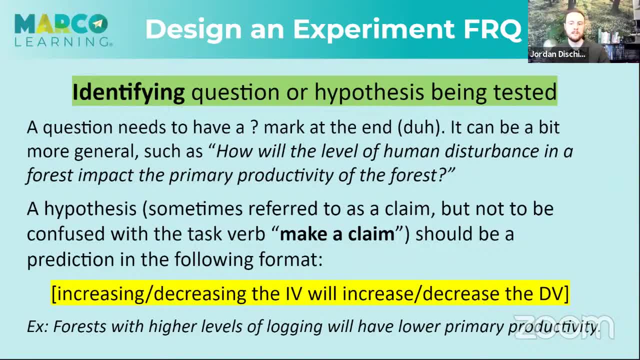 IV independent variable will decrease or increase the DV And so an example here: forest with higher levels of logging will have lower primary productivity. So it's really simple. You don't need to go into because you don't need to go into justification, you just need to simply give it in. 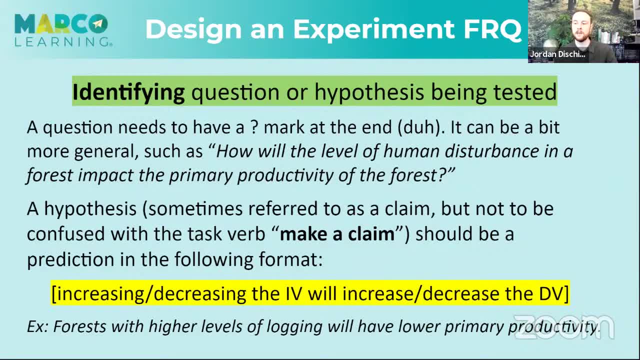 this format. So you don't want to say forest with higher level of logging will be unstable or will be unhealthy or will be unnatural. Those aren't things we can measure. We can't look at a forest and say how unstable is it? Seven units of instability. You know we don't have a dependent variable there. 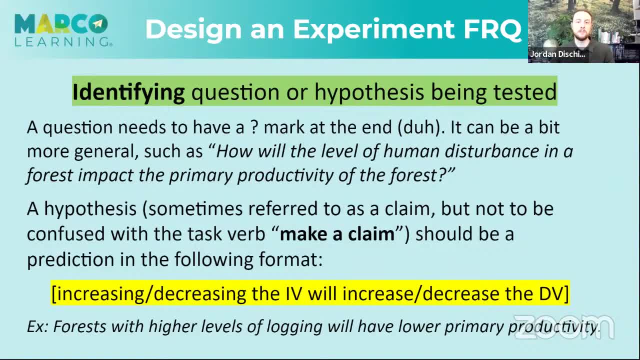 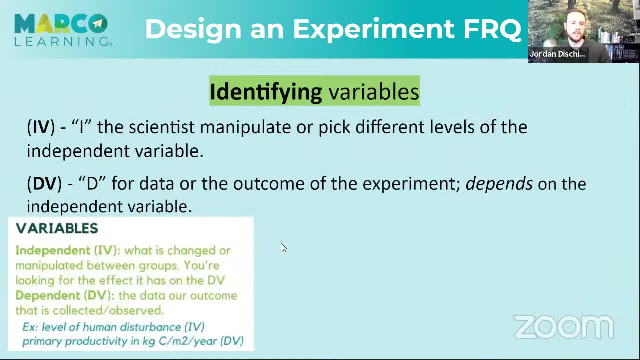 but if we say primary productivity, all of a sudden we're talking about something very specific. you know, kilograms of carbon biomass added per year, per meter squared, That's a direct unit of primary productivity. So make your dependent variable clear. The second thing you may 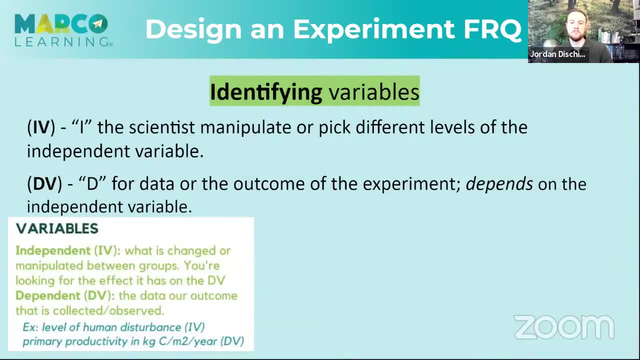 be asked to do is identify variables. If you're identifying variables, remember that IV, I, the scientist, manipulate or pick a different level of the independent variable. So it's what you're changing between each group. It's what I manipulate, I pick. you know how much carbon. 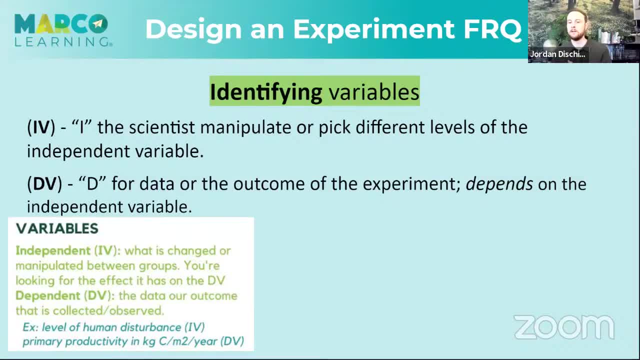 dioxide goes into this tank or I pick. you know how high the level of human disturbance is in different forests I might be looking at for their productivity. DV, I like to remember the D stands for data, And so it's the outcome of the experiment and it depends on the independent variable. 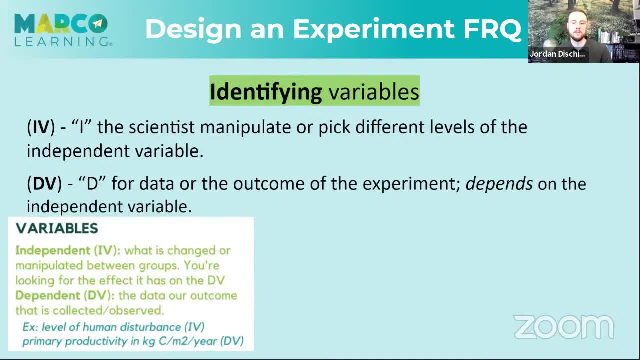 So the dependent variable in this case is productivity. The primary productivity of a forest depends on the level of human disturbance- how much is being logged, whether or not there are hikers or bikers, And so I really recommend trying to commit this to memory so that when you have to, 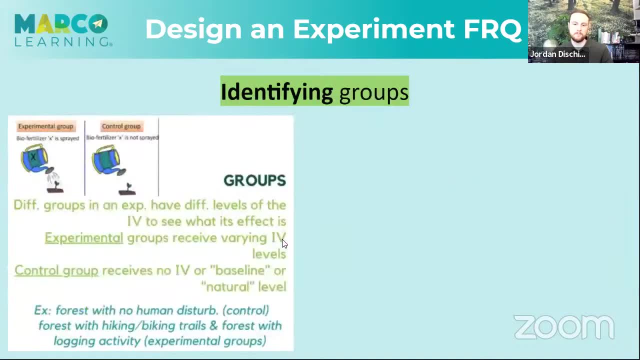 identify variables. it's an easier thing for you to do When we get into identifying groups. groups are different ways that you're going to do the experiment, And so you might have an experimental group which, if you're measuring pesticides, gets a certain concentration of the pesticide, whereas a control group would not receive that pesticide or that fertilizer. 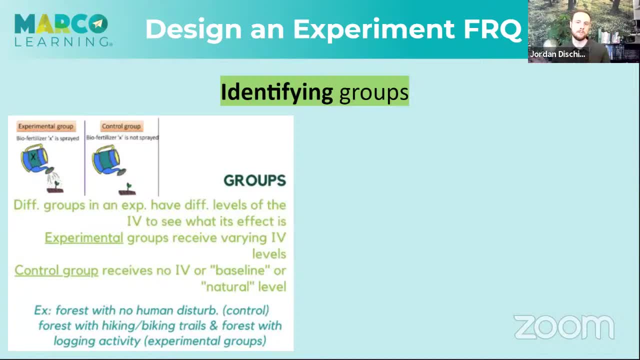 So it's held in a natural state. It doesn't receive varying levels of the independent variable. If we're talking about this forest example that I've started using, you know a forest with no human disturbance, So humans are not biking, hiking, they're not logging. That would be a control, That would be the background level of productivity. that goes on just naturally, normally. 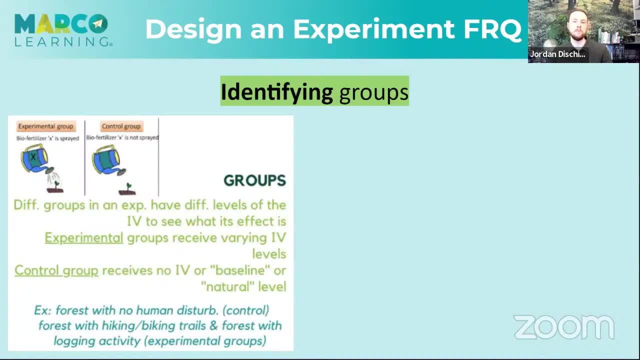 And we need that as a baseline or as a comparison. Then we might have our experimental groups. be a forest with hiking and biking trails and another forest with logging, Or maybe one of the forests is clear cut and one of them is selectively cut. Those are different levels or concentrations or extremes of. 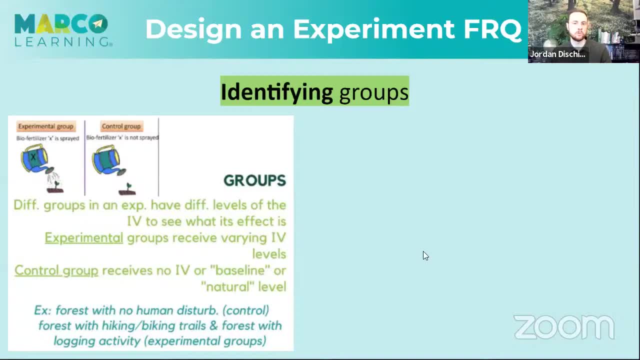 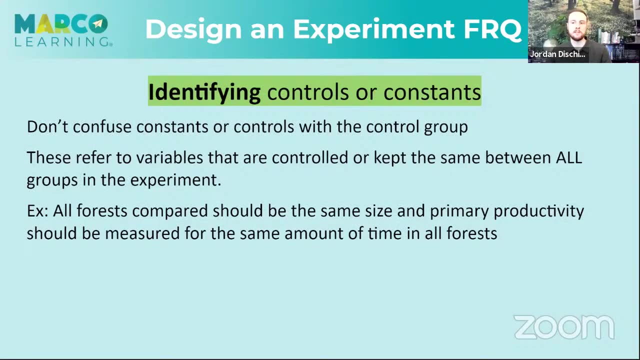 the independent variable, which is disturbance. So again, really important- you have a control and at least two experimentals. If you have to identify controls or constants, don't get confused and think this is a control group. They will ask you specifically with the word group if you need to identify a group, But if they're just asking you to identify controls or constants, these are variables that are held. 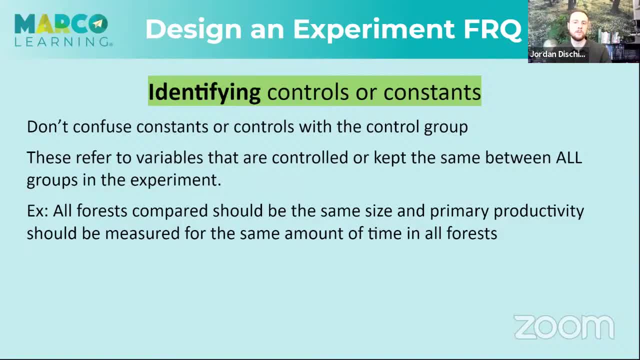 basically stable, constant throughout all the experiments. And so, for example, you know, all Forests should be compared to the same size forest. You're not going to compare one forest that's 100 acres and another forest that's 10,000 acres. 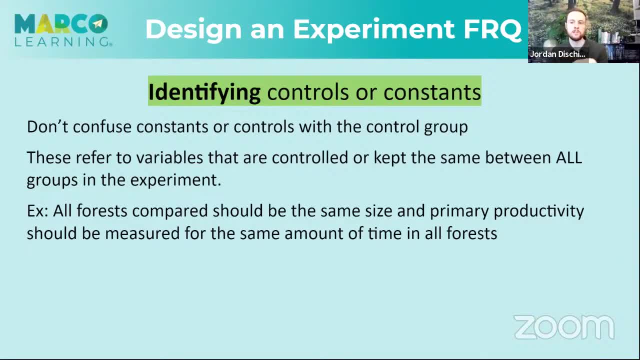 That's not holding your variables constant. So you want to compare forests of the same size and you'd want to measure primary productivity in them for the same amount of time. You wouldn't want to measure how productive one was for a year, but only measure how productive another one was for a month. 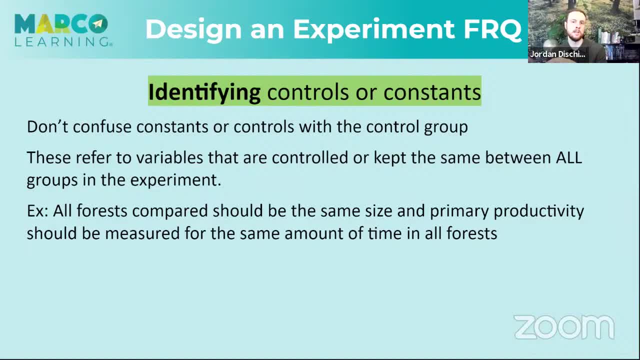 So think of it as things that you need to do the same between each experiment so that you're not adding in different variables. You only have one independent variable. only one thing changes. Everything else needs to be a control or a constant and be held at a stable state. 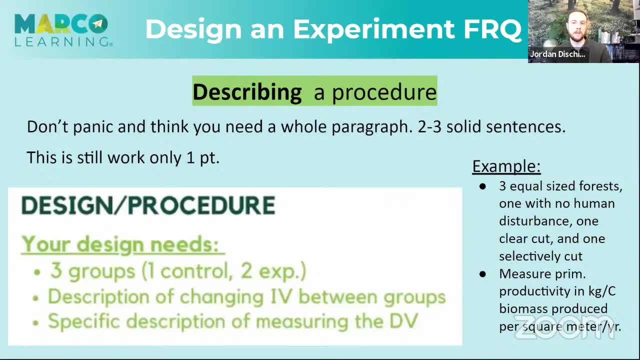 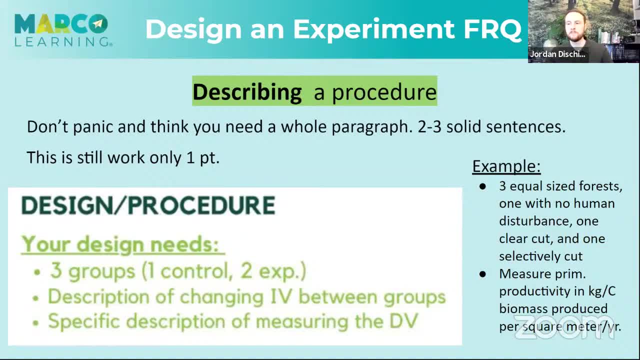 You don't need to do that. Just keep it simple: Two to three sentences and what you want to do to make sure you're earning. the point is three things: Identify that there will be at least three groups. Identify that there will be one control and two experimental. and then you need to say how was the independent variable changed in those experimental groups? 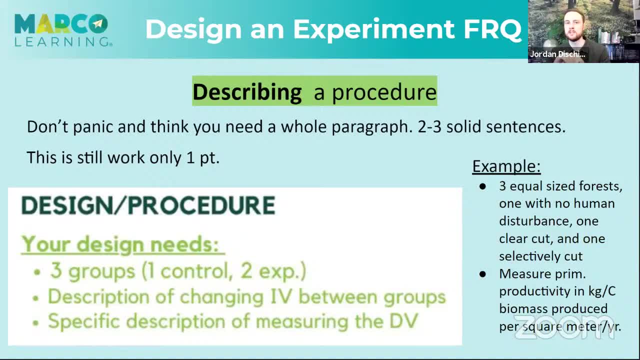 And then, finally, you need a specific description of measuring the DB. So how will the dependent variable be measured? How will the data be gathered? So, for an example, this would be a fine procedure if i wrote this out in full sentences- for this forest disturbance. 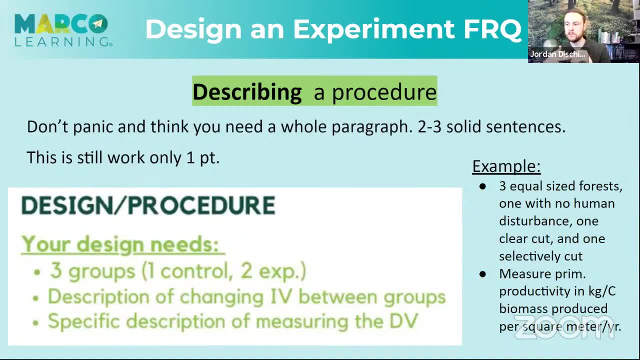 frp three equal size forests: one with no human disturbance- that's our control- and then one that's clear cut and one that's selectively cut. those are different levels of disturbance. clear cut is very high disturbance. selective cutting is lower disturbance. notice how we have control: no cutting. 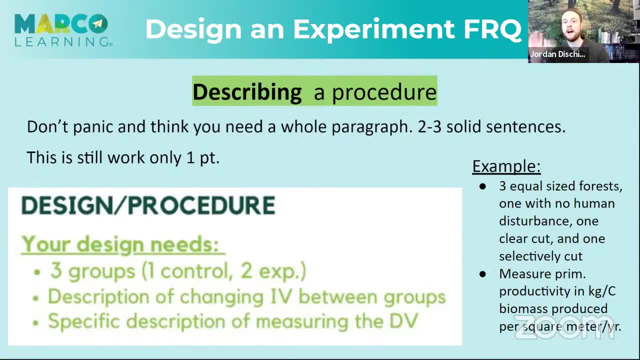 you know, medium disturbance, selective cutting, high disturbance, clear. and then the final thing is we need to clarify how are these data being gathered, and that's measuring primary productivity in kilograms of carbon biomass added per square meter per year. so we're going to measure out a square meter of each of these forests, measure how much carbon biomass is added to it in a year. 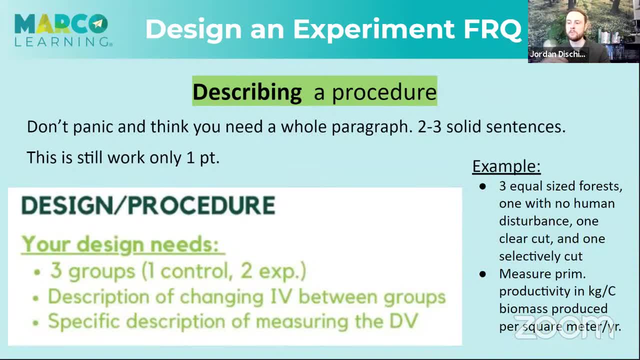 that will tell us how productive the forest is. now we probably want more than just one square meter. we probably want a handful, but we're going to measure how much carbon biomass is added to it. you understand the basic idea here. we have a clear dependent variable, clear data being gathered. 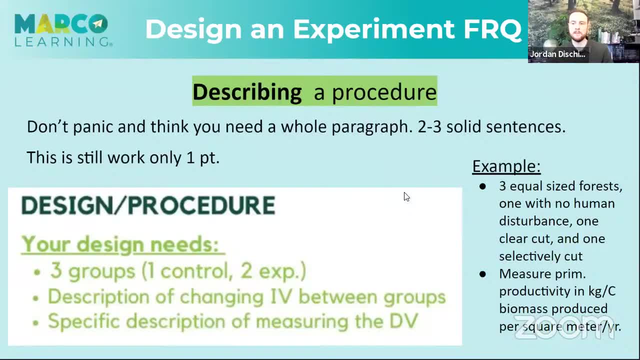 and that's enough for a procedure. it doesn't need to be a paragraph, it doesn't need to be. you know, gather all these materials, very simple groups, make sure you have a controlling experimental, make sure you say how the iv is different between the experimentals, and then give. 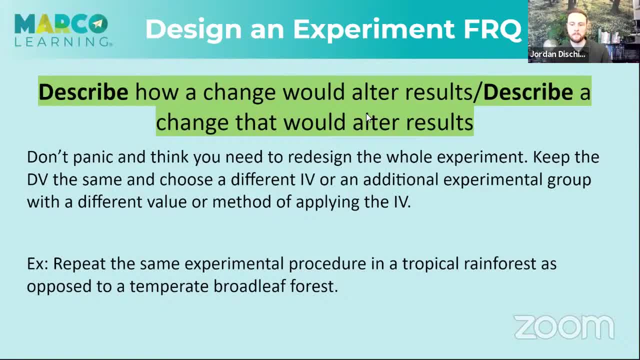 the db. okay, this is the trickiest part. this is the question on frqs about experiments that i see students miss the most. describe how a change would alter the results of an experiment. describe a change that would alter the results. so they may give you a change and say how would this affect the experiment, or they may 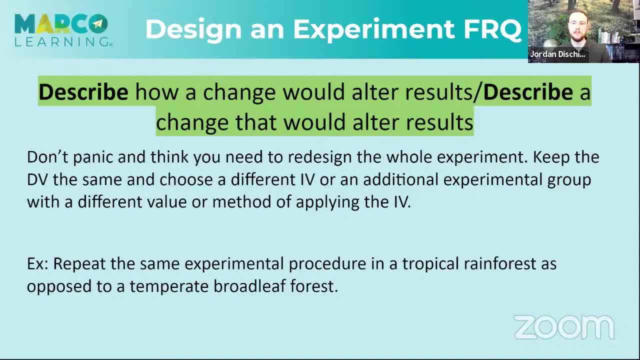 say, you pick a change and describe how it would alter the results, and it can throw students for a loop. sometimes they can kind of be like what like you designed this experiment, why am i remaking this experiment? but what they want to see is if you understand how changing an 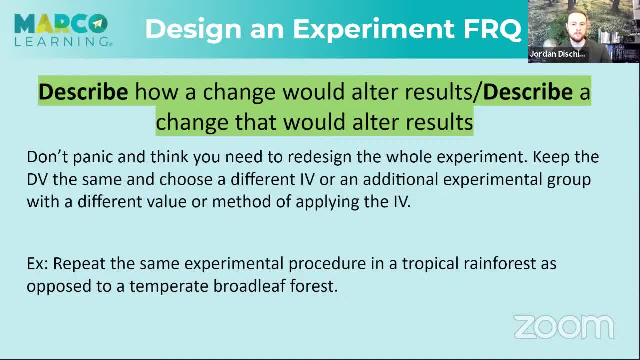 independent variable or manipulating an experiment will give you different results. so don't panic, don't redesign the whole experiment. keep the dv the same, so don't change what you're measuring. keep measuring- in this case productivity- but change the iv. pick a slightly different independent variable or add an additional. 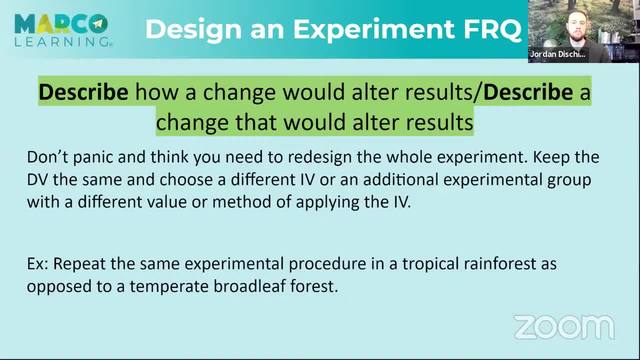 experimental group that has a different value or different method of applying the independent variable. great example here is: repeat the same experimental procedure that we've been talking about now you can add a, b in this particular experiment again. so the solution would be now, before you create an experiment, had you, had you added a system where you would 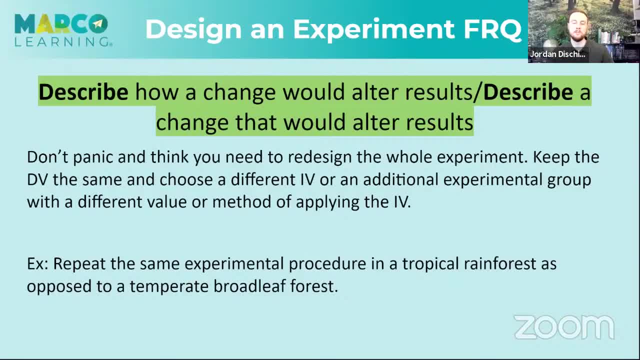 inform the package in silоль for the university ofまた c, ca feed data will take care of testing the fields based on what i've just talked about. so i'll combine both of those- a successful either or not successful fitch or whatever- to do- and we'll be using class as an exampleore's. which is this generalêso, and we're, you know, kind of taking the class runtime from each other and what they're doing within class. is you kind of jumping like because we have different project? Sabbator, which is what's the condition, where they're learning most of the questions and we're 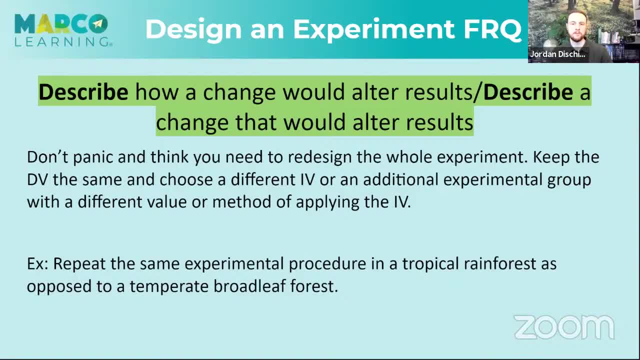 is has been like adding crushed limestone to kind of buffer the ph results, or like altering the temperature of you know tanks to alter how much you know carbon dioxide uh can, can move in or out. so you just want to pay attention to things that are common apes, you know vocabulary, common aids. 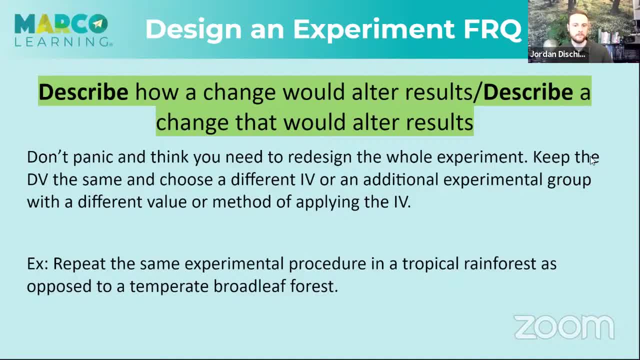 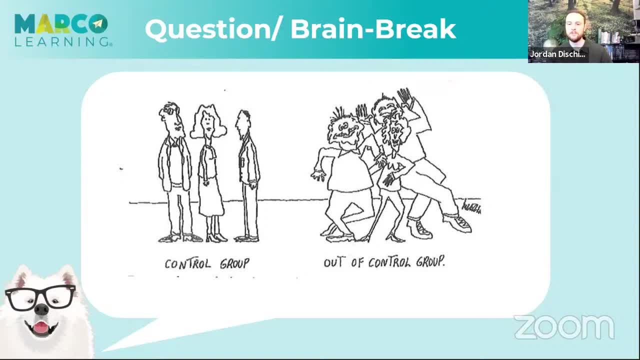 ideas that, may you know, appear on frq. so, uh, when we look at the control group, here we have a little bit of a joke and a brain break. here we have the control group who are just kind of chilling, and then the out of control group that are going crazy. um, so kind of a joke. that's your experimental. 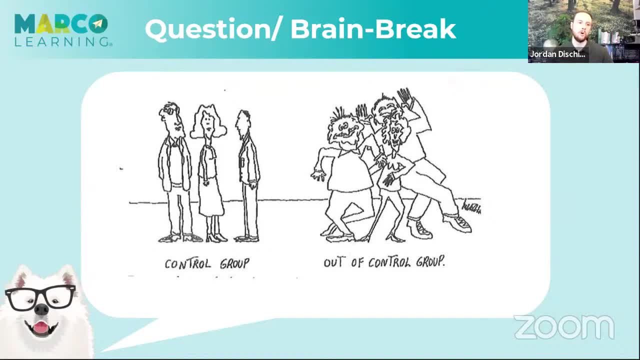 group over on the out of control. but remember, you always need a control group, you always need a chance to have something serve as a comparison. so i'm just going to take a brief break here to grab a drink of water and then we're going to go on with content review for unit 7.. 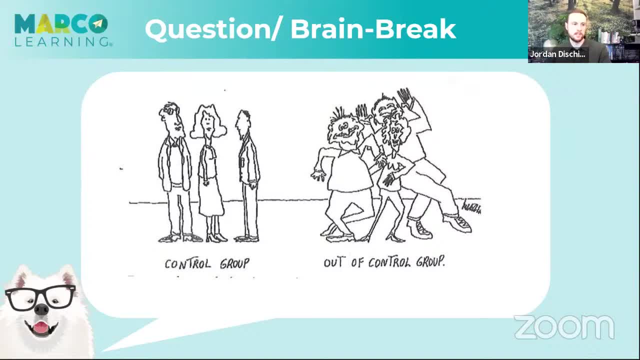 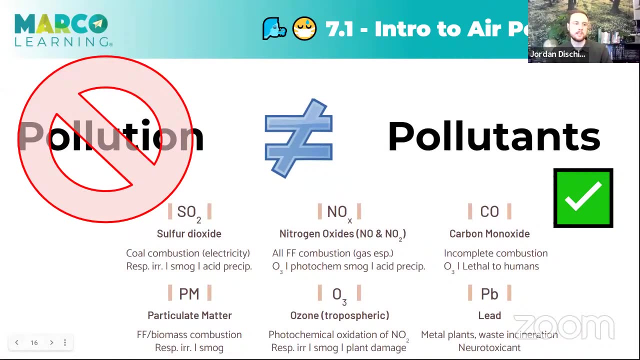 so let's go ahead and take a look at the comments. to ag good to see you in the comments, as always, and um, all right, so let's go into our review of unit 7 now. so unit 7 is air pollution, and it's really important that we know the difference between pollution and pollutants. so pollution: 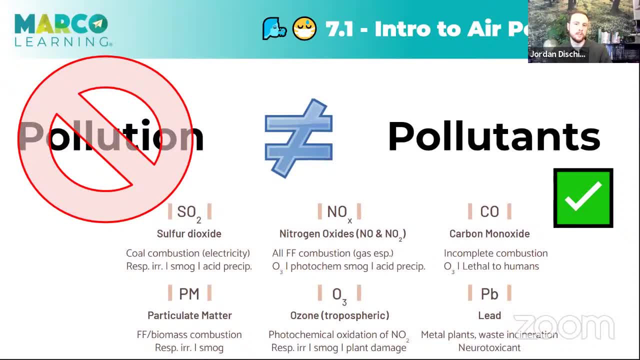 is going to be a vague idea that's never going to earn you points on an frq. it's just too vague, it doesn't really mean anything. specific pollutants, on the other hand, are specific chemical compounds, and we have six here that you should know. that have clear. 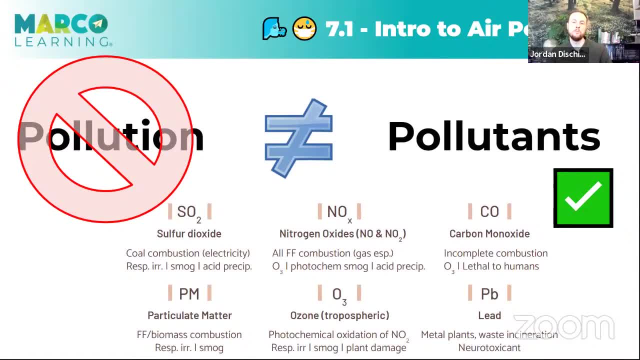 sources and clear effects. so again, you want to strike the word pollution from your h vocab. it's an idea, it's not a specific thing. it's probably never going to earn you points on an frq. so the reason that i have these six pollutants on the screen is because these are the six pollutants that are regulated by the clean. 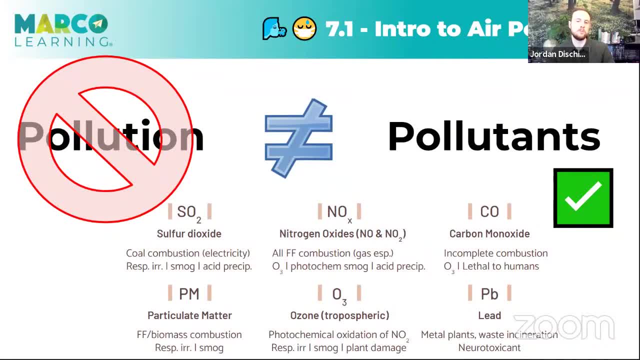 air act. so these are six pollutants that have direct sources, that can be regulated by the epa and that have consequences for their pollutants. we have so2, sulfur dioxide, that comes primarily from coal combustion, especially for electricity, and then you should know that it can be a 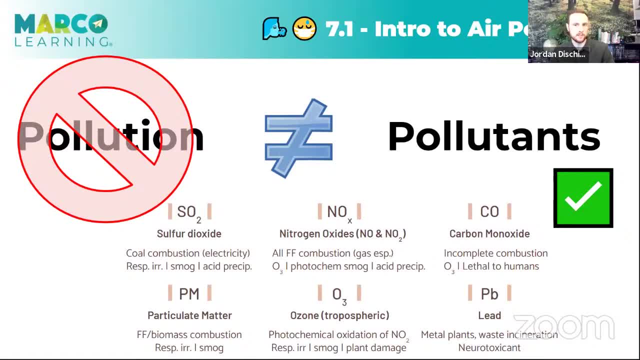 respiratory irritant. it can be a precursor to sulfurous smog and it can form acid precipitation. we have nox, which refers to the term nitrogen oxides. that can be no or no2. this comes from all fossil fuel combustion, but especially gasoline vehicles. so car exhaust is like the number one. 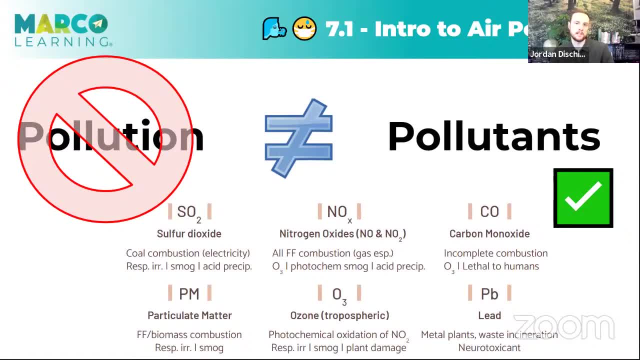 source of nox. it can form ozone. we'll talk about why that's important in a second. it can form photochemical smog and it can form acid precipitation. so socks and nox are two big air pollutants that you should be familiar with. then we have carbon monoxide, not carbon dioxide, carbon. 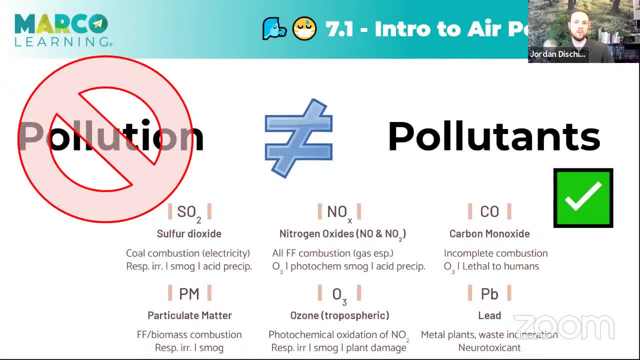 monoxide comes from incomplete combustion. so when a substance does not burn all the way, especially in a furnace, or we're talking about biomass, and that can form ozone, but it can also be lethal to humans. we'll talk about why in a bit. then we have particulate matter. this is a great go-to air. 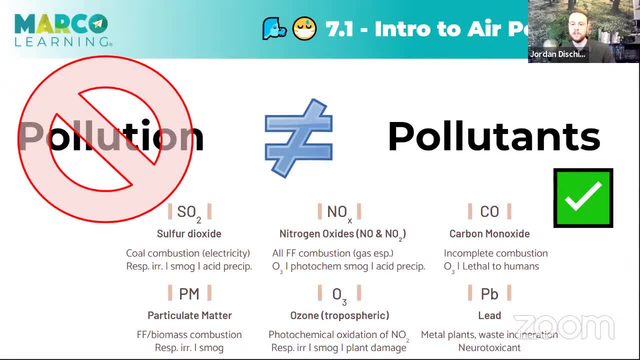 pollutant if your brain is fried and you're at the end of an frq and you're like: shoot. i don't have a good air pollutant in this question that's asking me about air pollution. go to particulate matter. pm- it's just a fancy word for a little bit of air pollution. it's just a fancy word for a little bit. 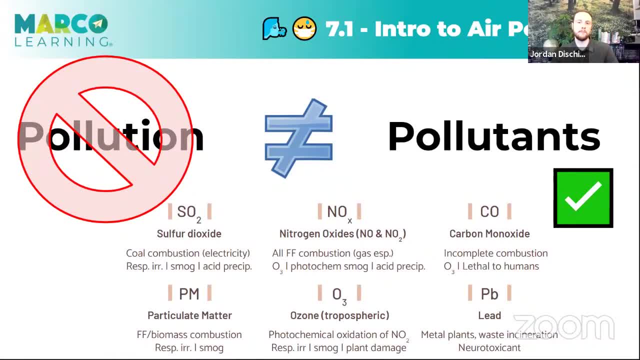 of matter that float around in the air, and they can come from any sort of combustion process- you know, construction, agriculture- and they can be respiratory irritants as well, so they can get into the human respiratory tract, damage it, but they can also help contribute smog. then we have. 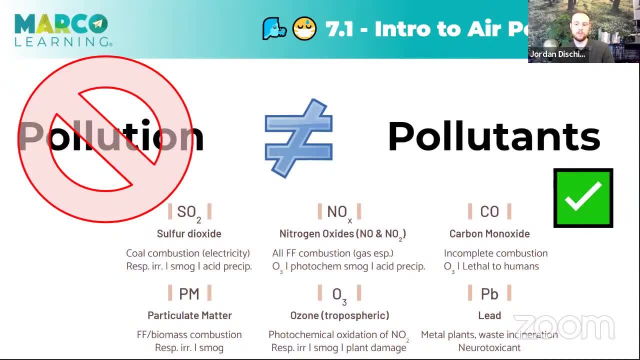 ozone or o3, now in the troposphere down near earth. it's very harmful. it is harmful to human respiratory tracts. it can damage plants, especially their stomata. it can help contribute to smog. i'm going to talk a little bit about nitrogen dioxide, so we need to know that it comes from no2, so it 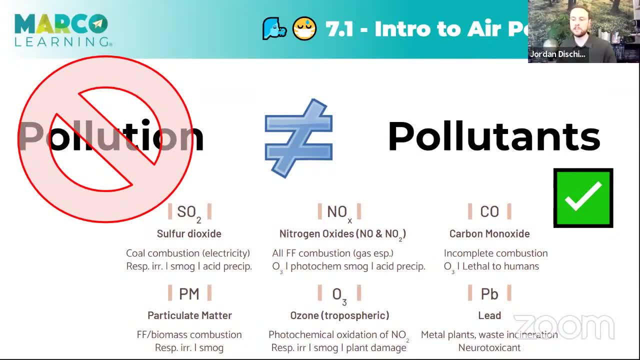 comes from when nitrogen dioxide is given off by car exhaust and then the sunlight breaks it down. we'll go through those steps in a second, and then finally we have lead. lead comes from, you know, metal manufacturing. it comes from waste incineration, especially burning medical waste, and then we 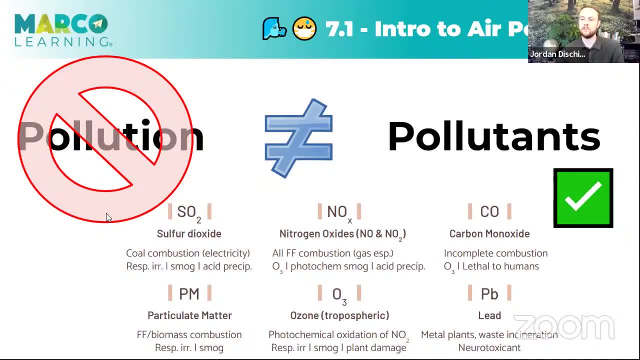 should know what the neurotoxicants. it's going to damage the central nervous system, especially the infants, and so if you're struggling with identifying specific pollutants, try to commit these sticks to memory. these are probably the six most important pollutants that we're going to talk about. 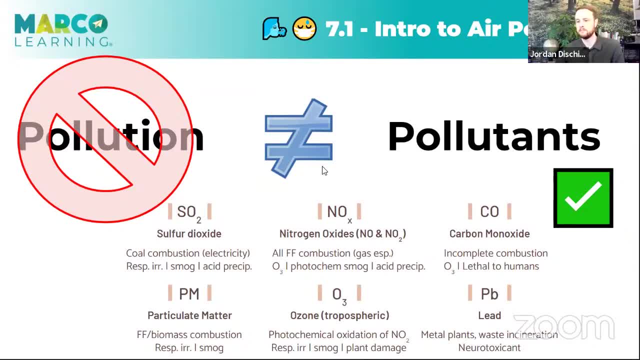 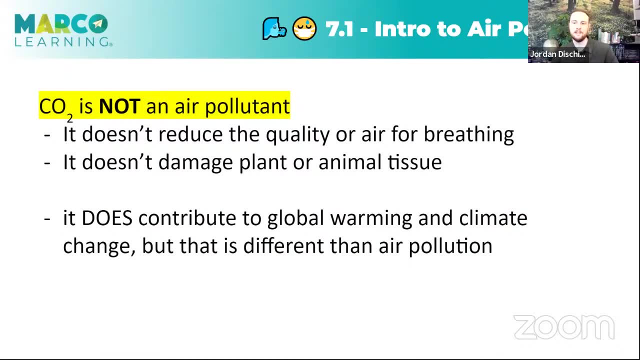 important air pollutants when we talk about unit 7.. noticeably absent from that list is co2. so carbon dioxide is not an air pollutant. i want to say that again. co2 is not an air pollutant. and you may be wondering why. because it is, you know, a compound. 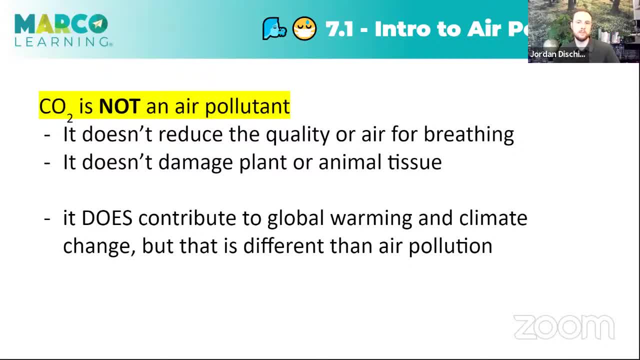 that we talk a lot about. when it comes to the atmosphere, it is a huge greenhouse gas. it's the most important greenhouse gas, so it does contribute to global warming, but it doesn't reduce the quality of air for human breathing or for life directly, and so it's not going to damage human. 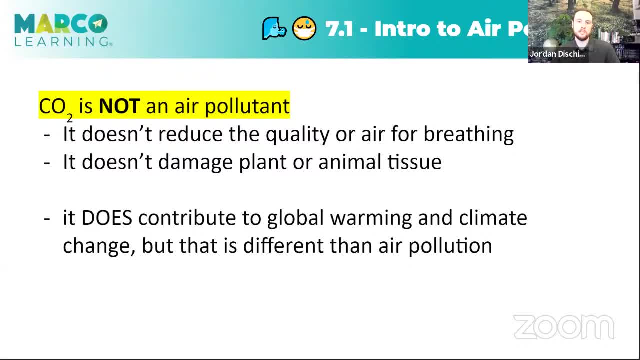 lungs. it's not going to damage plant tissue. um, what's interesting is the supreme court is actually litigating or going through the process of a lawsuit to determine whether or not co2 can be regulated by the government. but it is not in the clean air act and so it is not considered. 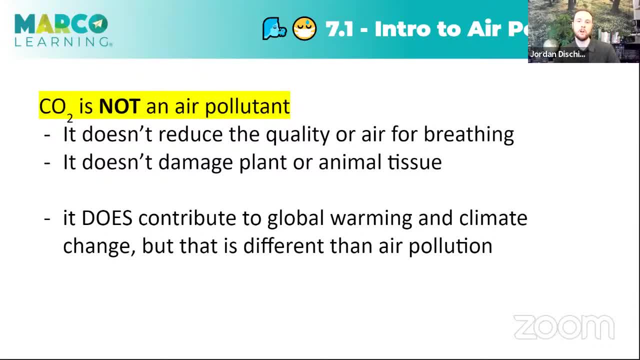 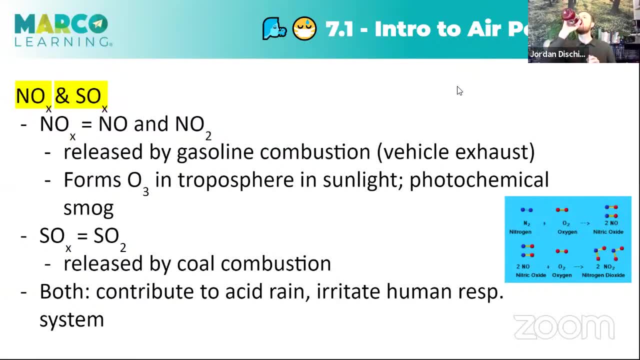 an air pollutant on hfrqs typically, so you want to steer clear of it when you're talking about air pollutants. if you're talking about air pollutants, you're going to want to keep in mind: right above co2 is co2 and on both sides, as i mentioned earlier, um sox and nox are two really important air pollutants. 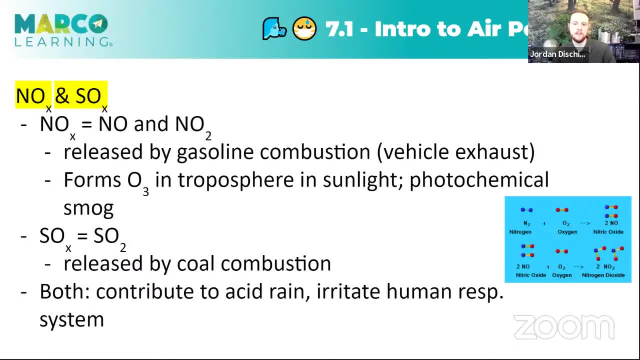 to understand. so nlx refers to both nitrogen oxide and nitrogen dioxide, no2. as i mentioned, these are going to be released primarily by gasoline combustion, so your car is going to give off a lot of nox and it's going to form a non-topological solution. so co2 is going to. 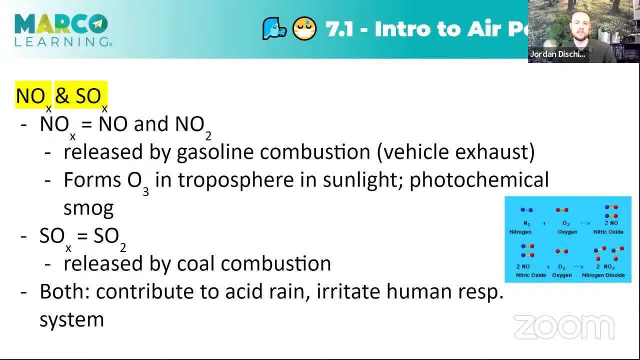 give off a lot of nox and with that, it's going to give off a lot of co2. this is a really important solution. that's what we're going to talk about next. all right, now we're going to talk about co2, but O3, or ozone in the troposphere. That's because the sunlight breaks it down into NO and O and. 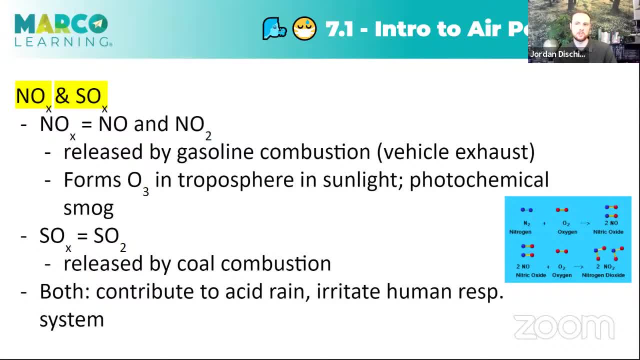 that free oxygen combines with O2.. We'll talk about those steps shortly. Then we have SOX, Now SOX. sometimes you use the subscript SOX, but it's safer. on FRQs, just to say SO2.. It's all for. 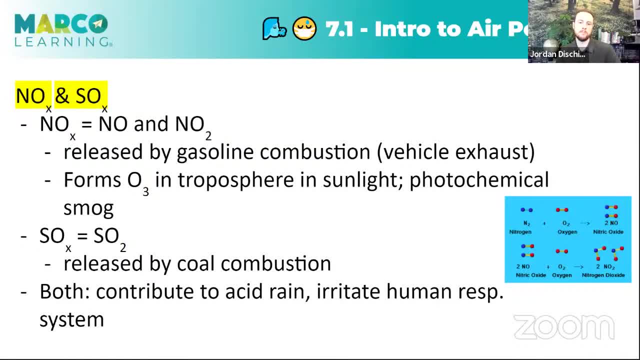 dioxide, because that's the primary air pollutant that we're talking about here, in this case SO2.. It's going to be released by coal combustion, primarily for electricity generation. We should know that both NOX and SOX contribute to acid rain and they both irritate the human respiratory. 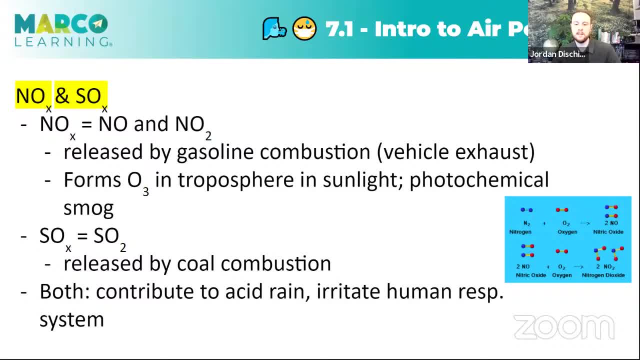 system. They're both going to damage eyes, lungs, things like that. They're both going to contribute to acid rain. I'm going to stop here for a second because I see a question in the chat. All right, Lauren, good question. 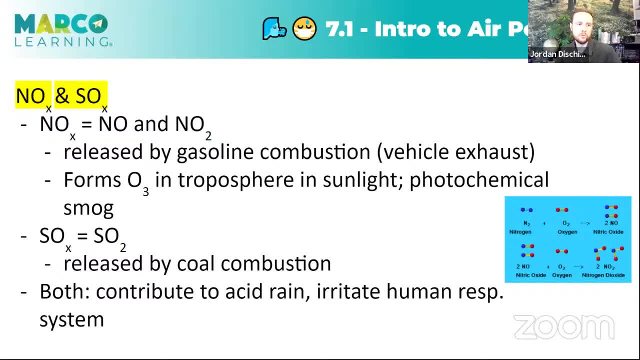 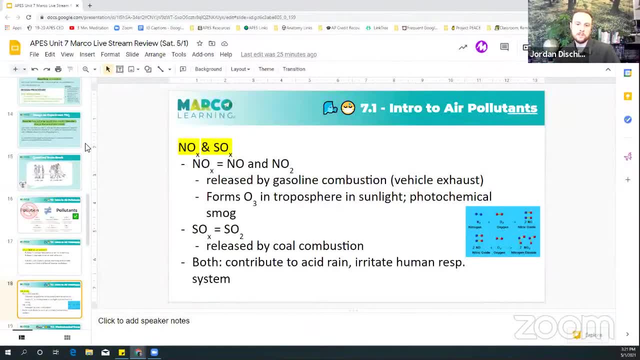 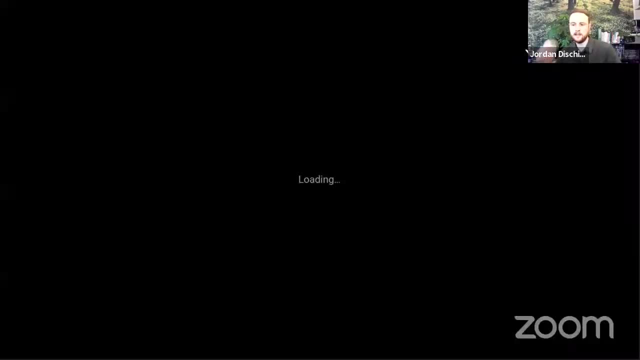 Lauren has asked if we can go through the difference between the control group and the constant and the types of FRQs. I'm going to pop back a couple slides to show you those, Lauren, so you can see them. If we look here at the three different FRQs, they're going to be describing 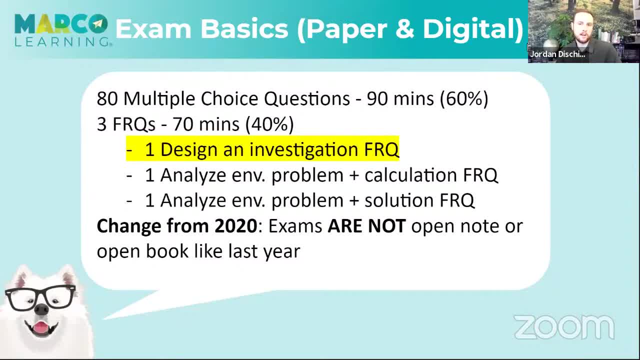 an environmental investigation. That's what we just covered in this video. You can see the replay on Market Learning's channel here shortly. Then we have analyze an environmental problem and do some math, some calculations. Then we have analyze an environmental problem and propose solutions. Now, Lauren, if you don't, 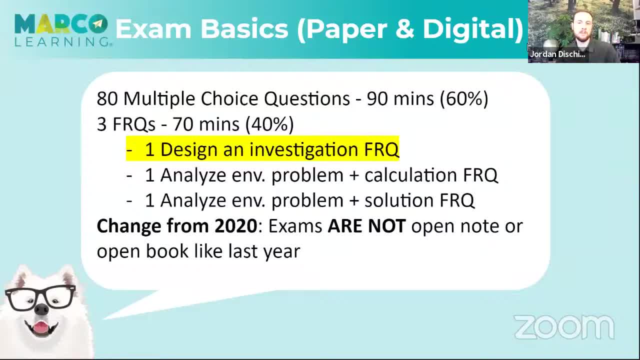 already subscribe to my channel. you want to make sure to do that, because I'm going to have an in-depth video for all three of these FRQs. I'll put my link tree in the comments here. Then you want to make sure that you go over and check out my channel, because I'm working on the first video. 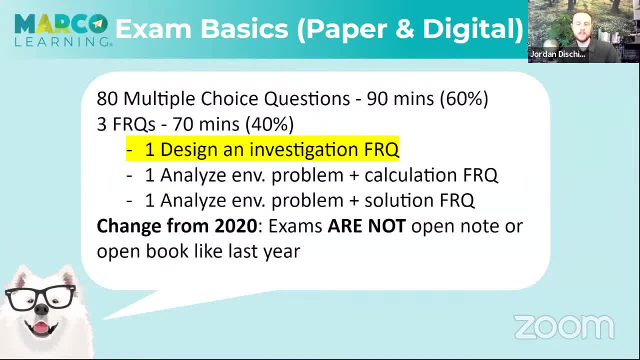 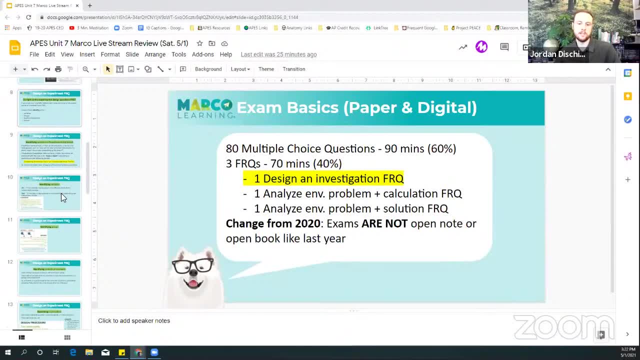 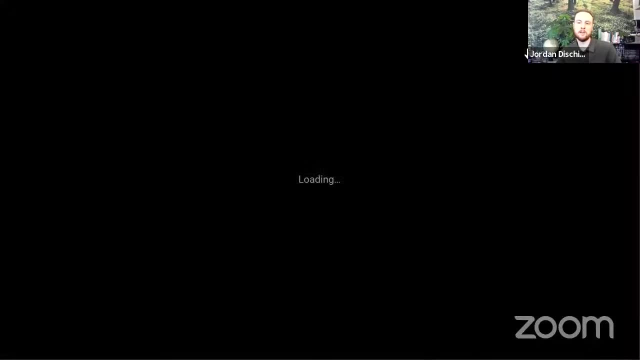 right now editing. It'll be done soon and posted soon. Then the other two videos will be coming out soon, but it'll go in-depth through each of these FRQs. Then for the control group and the controls or constants, the control group is going to be what you are basically. 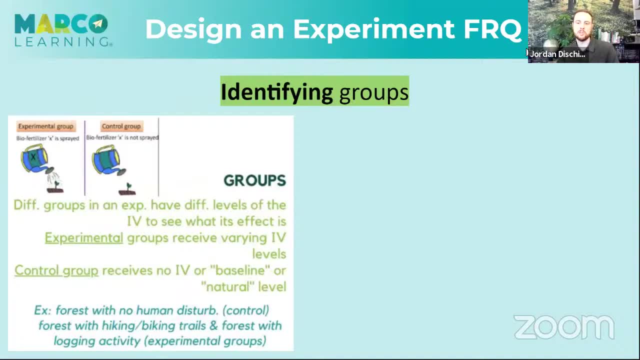 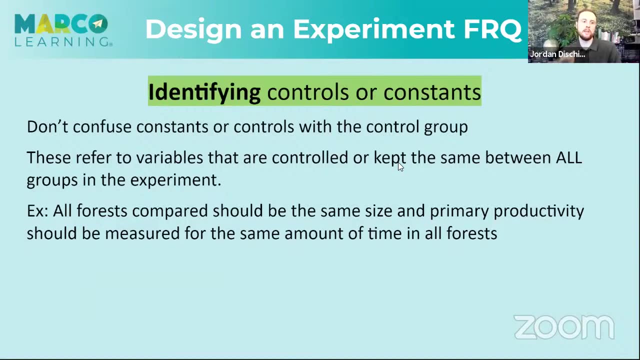 using to compare to the other groups. It's going to be one way of doing the experiment. If you're asked to identify a control or a constant, on the other hand it's just saying a variable that doesn't change between the groups. so different things. One of them is a way of doing. 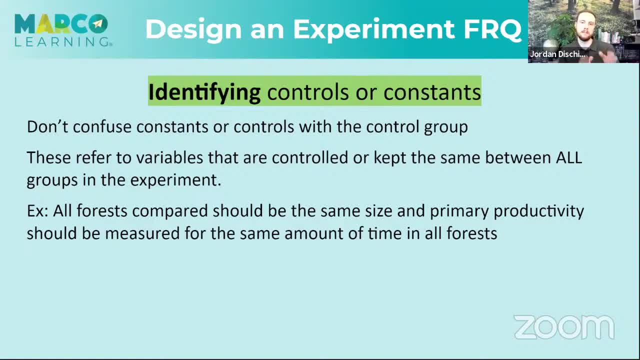 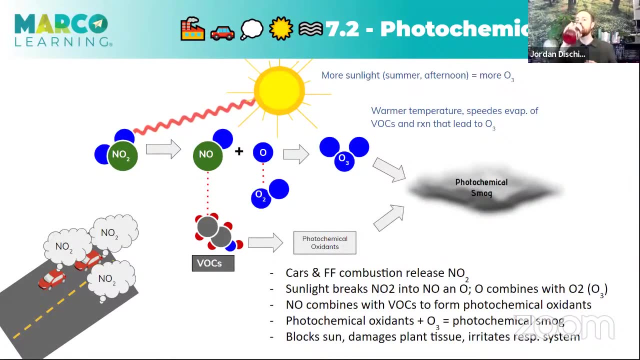 the experiment where you don't have the independent variable applied control group and the controls or constants are things that you keep the same between all groups of the experiment. Hopefully that was helpful. Luke V disgu вход. I will share my link tree in the comments here. I don't think it will actually pop up as a link. 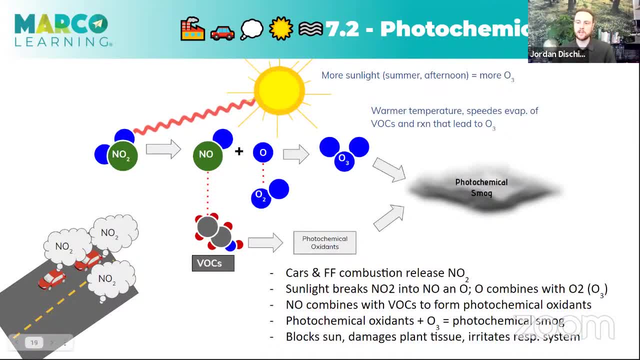 but you should be able to copy and paste that. still Another topic that we definitely need to understand- Luke V disgu eruption from one 2.3s Steps to understanding Essex BCES is: they would love to understand what you would like Belmont CSU to do when you want to apply a first test in a 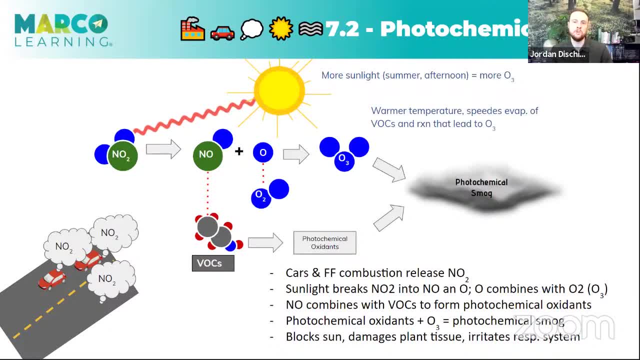 is 7.2 here: photochemical smog. So you should be familiar with the chemistry of how photochemical smog forms. So the way it forms is NO2 is released, actually by vehicles. Now it can come from, you know, coal combustion as well, somewhat natural gas a little bit, but primarily it's. 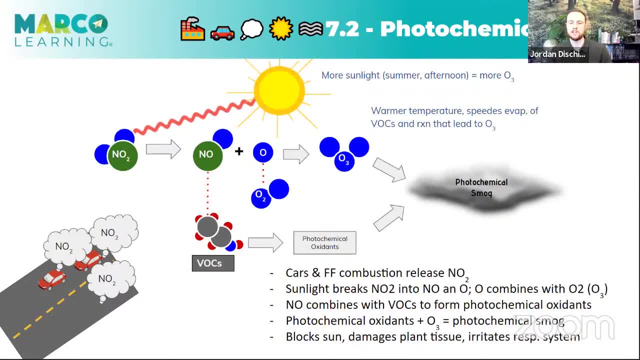 coming from our exhaust vehicles And so that NO2 goes up into the atmosphere. Then what happens is the sunlight breaks NO2 down, So you can see that red squiggly line hitting the NO2.. Now it's just nitrogen oxide, NO and O, And that free oxygen is going to combine with O2 in the atmosphere. 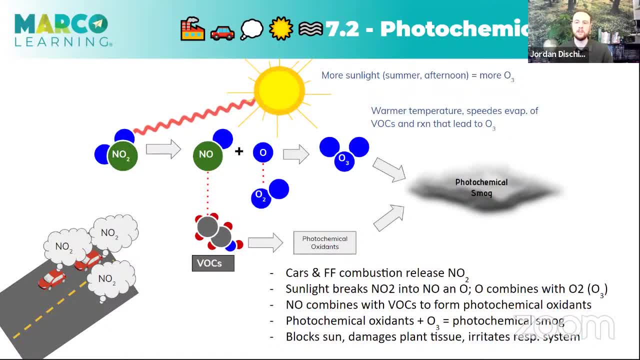 and it's going to combine to form O3, and that's ozone. Now normally this process just reverses and the ozone breaks down to form O2, and the O goes back to NO2.. But when you have VOX present, 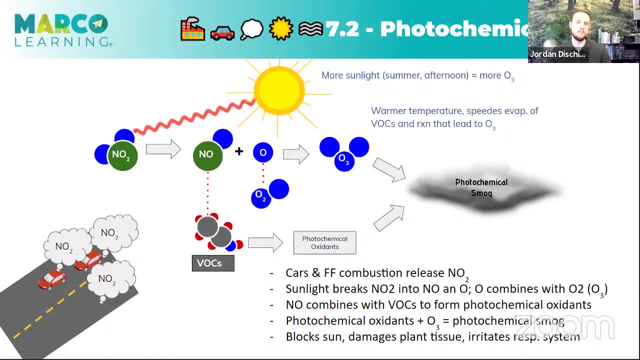 volatile organic compounds. these are things like gasoline emissions from you know gas stations. some laundromats emit VOX. a lot of you know petrochemical or plastic manufacturing industries emit VOX. They're going to bind with NO And VOX and NO combined. 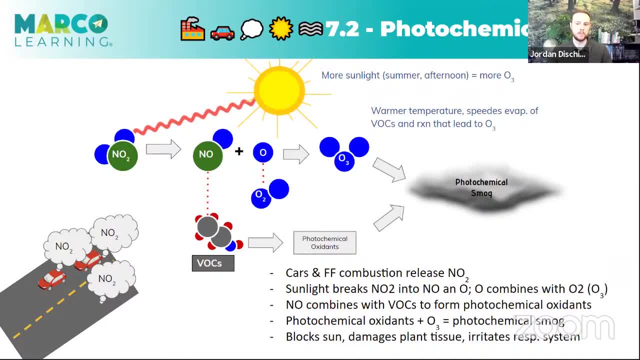 form a big class of compounds that are called photochemical oxidants. So with those VOX present they bind to that. NO, Now we don't have the breakdown of ozone. Instead we have the photochemical oxidants combining with the ozone and we get photochemical. 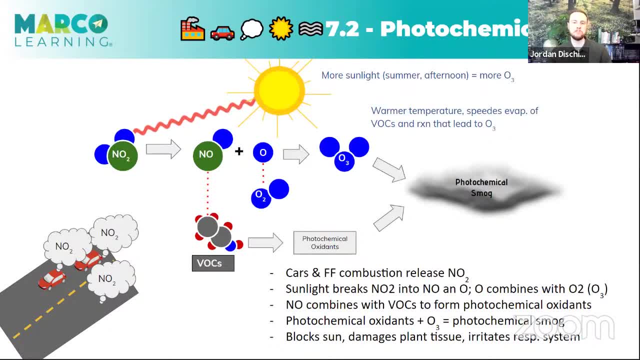 smog. So that's a big class of compounds that are called photochemical oxidants. The problem with photochemical smog is it damages plant tissue. It can reduce the rate of photosynthesis. The ozone in photochemical smog can damage plants directly and it can irritate. 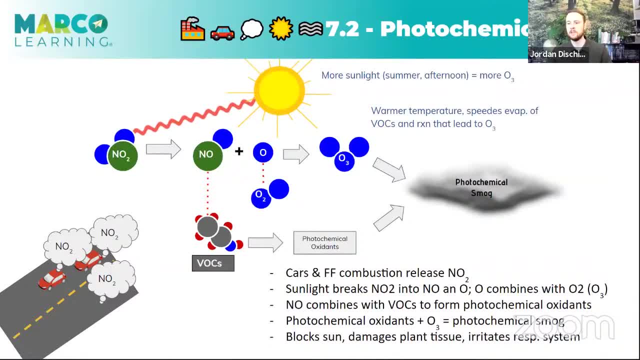 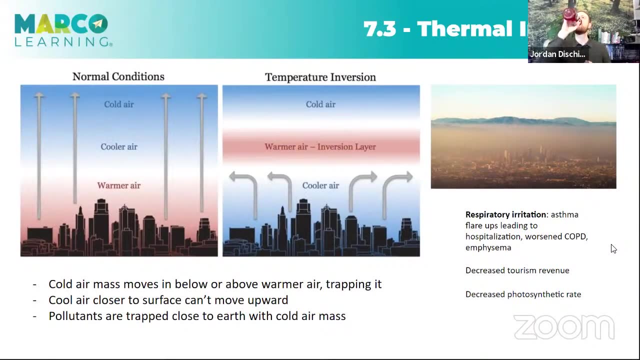 human respiratory systems make it harder for humans to breathe. It can make it harder for humans to see, And so there's a lot of issues that happen when you have photochemical smog formation. Next we have a thermal inversion. So in a thermal inversion it's kind of a tricky concept to 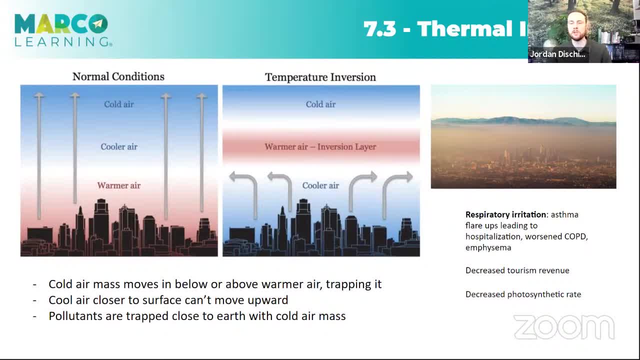 understand. So we're going to work on the normal conditions first and then we're going to go to the temperature inversion. So normally, warm air rises and as it rises it cools and it expands and becomes less dense, And so what that's going to do is carry pollutants away from the surface of 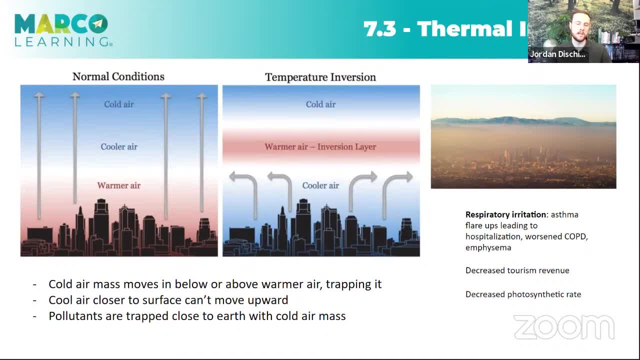 Earth, And so what that's going to do is carry pollutants away from the surface of Earth, And so under normal conditions, we have this warm air rising, cooling and expanding and it helps kind of lift pollutants that are produced at the surface. You know things like 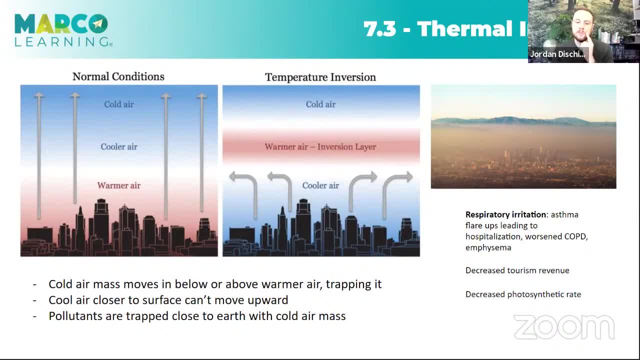 particulate matter, carbon monoxide from cars, NO2 from cars, helps lift it away from the city In a thermal inversion or a temperature inversion. what happens is a cold air mass moves in very quickly And it can basically sweep in below the warmer air mass. And now 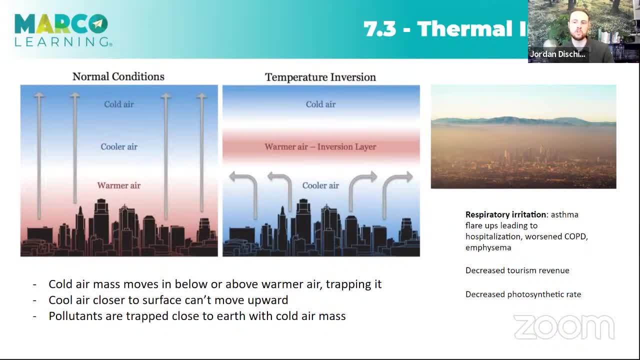 there's a less dense air mass of warm air above it, but it's trapped beneath the cold air above it And then the cooler air down near the surface is more dense and so it can't move up through that warm air mass And it traps these pollutants near Earth and it forms this, basically a blanket that. 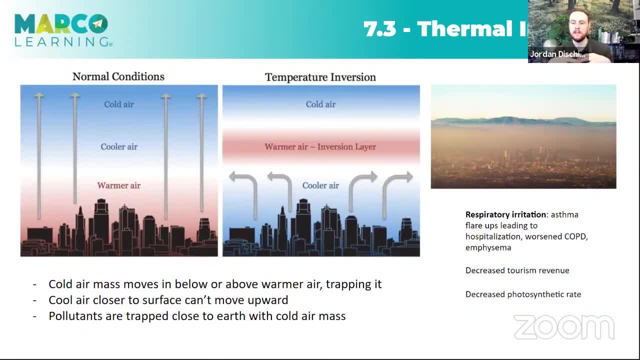 insulates and keeps all of the pollutants near Earth, And so this can happen a lot of times when you have a mountain range that doesn't really let the sun or the wind come in and disperse the pollutants, It can happen when you're close to the ground, And so when you have a mountain range, 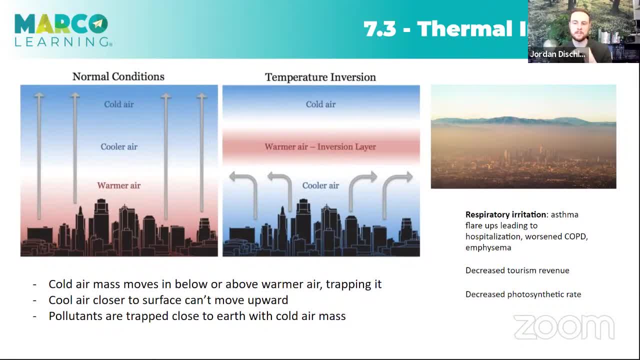 and a cold sea breeze moves in really quickly and traps that warm air between the cold air mass above and, you know, cold air mass below, And so this is going to be a big problem, as you can see in this picture, because now we have this really thick blanket of pollutants trapped super down. 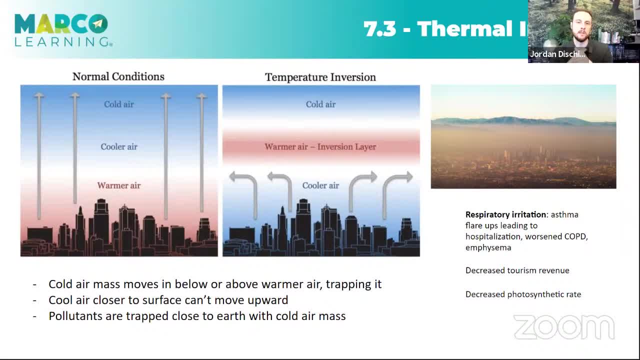 close to Earth, And so this is going to do things like make people's asthma worse, make COPD worse, give people emphysema flare-ups, And so it doesn't directly cause respiratory problems, but it can cause respiratory problems And so it can cause. 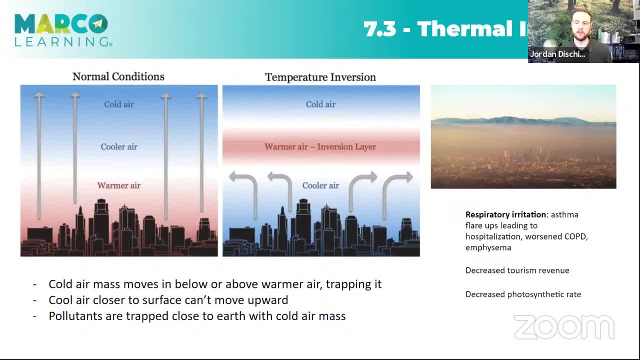 respiratory diseases like. it just makes them worse. It could make your asthma flare-up. You have to go to the emergency room, So that's a problem. It can also decrease tourism revenue- wow, revenue, because if you look at this picture, I mean who wants to go to this city and see this? 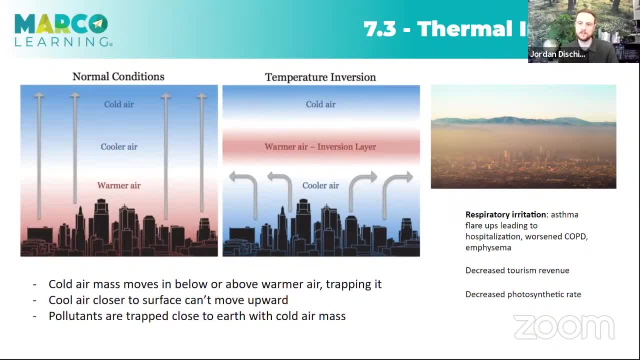 site. And then, of course, if you're a plant, you're concerned because there's not as much sunlight getting through, And so it's going to decrease the photosynthetic rate. So thermal inversions are an important concept to be on there. 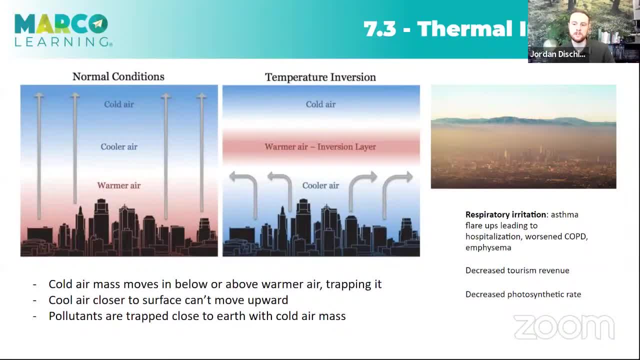 Able to understand. you should be able to look at a diagram and sort of understand what's going on If you see, like again, a cold ocean breeze coming in that could contribute to this- And it's going to be, you know, trapping that cold air close to Earth's surface. 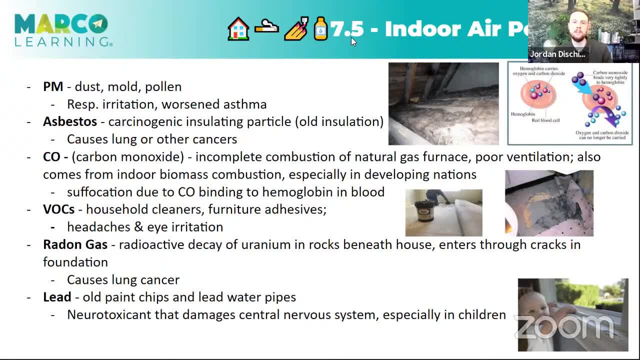 Okay, now we're going to go through some really important indoor air pollutants. So indoor air pollutants are pollutants that form indoors, as their name implies, And they can be really common, everyday things that exist in every home, Or they can be really. 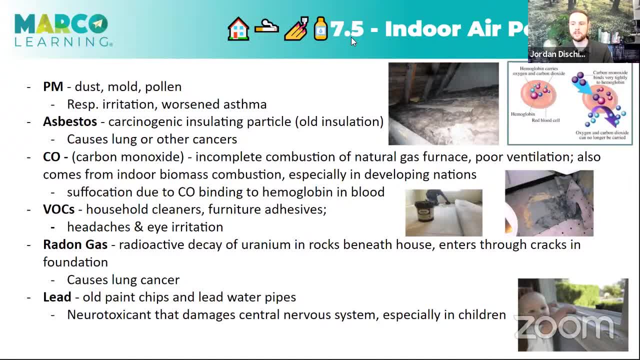 serious, you know, carcinogenic or cancer-causing things that come from some resources. So we'll talk through them here. One indoor air pollutant is particulate matter. Now, this could be anything like dust, mold or pollen, And this is going to get into human respiratory systems. 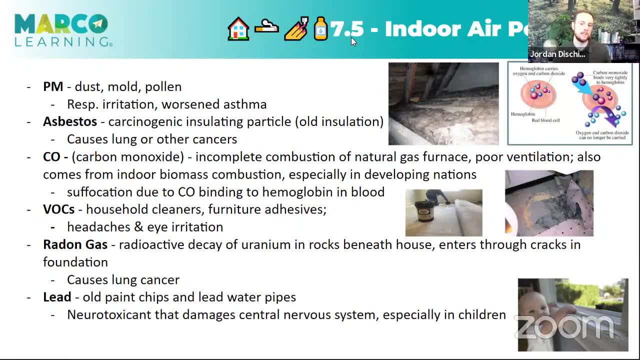 irritate those respiratory systems And again worsen asthma. get in people's eyes, It can give you a headache. So there's a lot of problems. if you have dust or mold in really high levels in your home, Then we have a really concerning air pollutant, which is asbestos. Asbestos comes from. 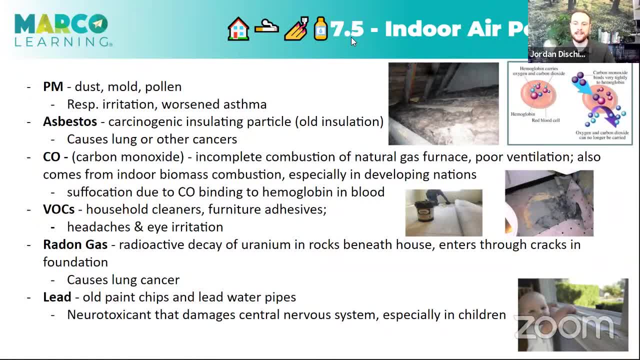 old insulation- So you can see a picture of it here- in an attic, And that insulation is going to give off these asbestos particles. They're thin, tiny little silicate particles, So they're almost like fiberglass And when you inhale them and they get into your lungs they can cause. 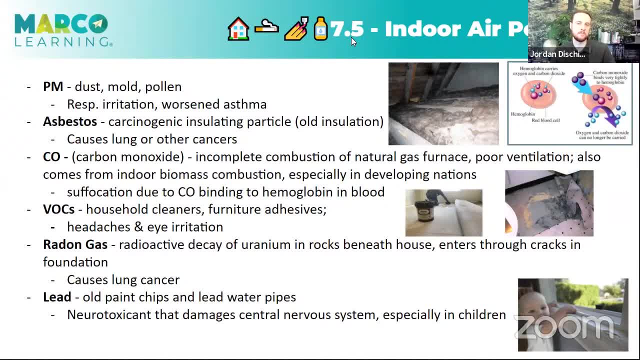 cancer, So they can trigger lung cancer but other types of cancer as well, And so to remove this, a trained professional with proper ventilating equipment should be removing this. So that's the key. You don't want to go do this yourself, You want to train professionally. Then we have carbon. 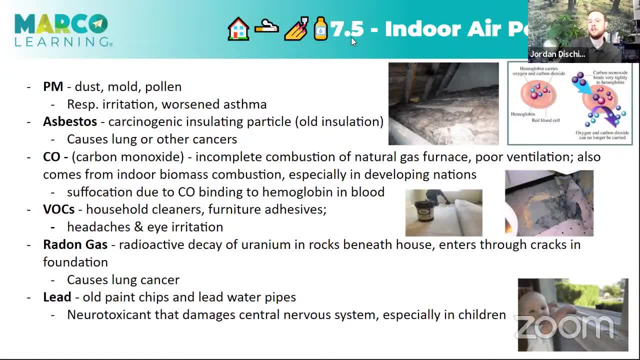 monoxide. As I mentioned earlier, carbon monoxide comes from incomplete combustion, So this could be a furnace. It could also be indoor biomass, If we're talking about a developing nation that uses a lot of wood or a lot of dried plant matter to cook. If you have poor ventilation, meaning 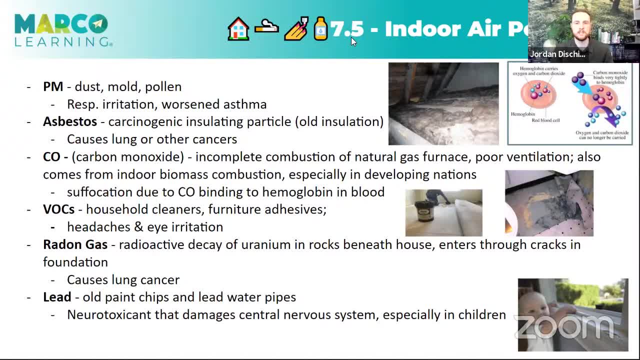 that your furnace is malfunctioning and it's releasing that gas into your home instead of outside. that could lead to carbon monoxide poisoning, which is where carbon monoxide gets inhaled into your body, goes into your bloodstream and then it binds with the hemoglobin. 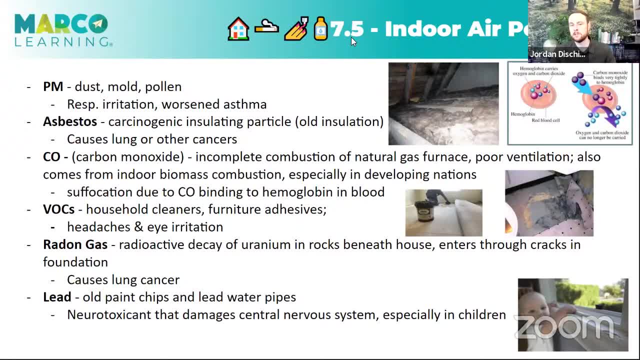 in your red blood cells. The problem with that is then your red blood cells can't bind to oxygen and you can suffocate and it can actually be lethal. So most homes have carbon monoxide detectors and they'll start to beep if carbon monoxide is detected, since it's odorless. 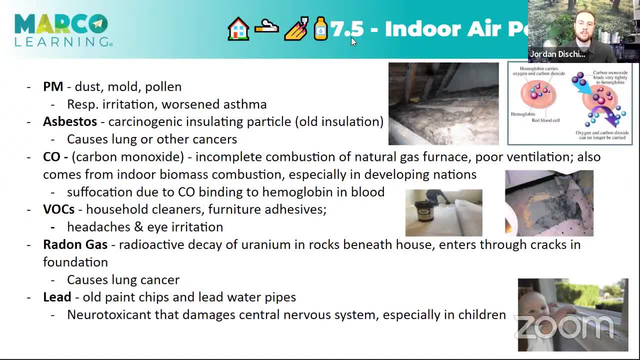 and you can't necessarily smell it. So really important to make sure you have a working carbon monoxide detector. In terms of how to fix that, you would just need a furnace repair to come and make sure it's not releasing those fumes in your home. Then we have VOCs. VOCs are volatile, organic. 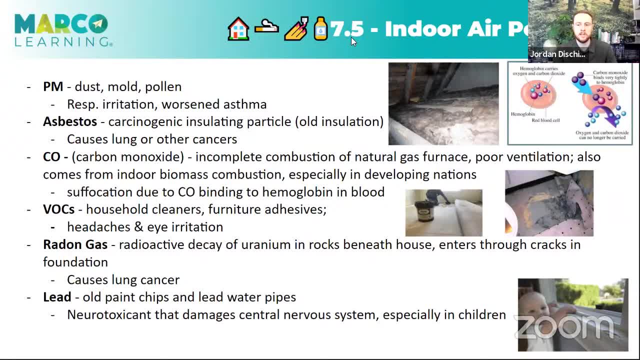 compounds, and these can come from everyday household cleaners. They can come from furniture adhesives- You can see this guy who's gluing down carpet- New homes, especially that smell of fresh carpet or fresh fabric or upholstery that a lot of times smells good, You may think. 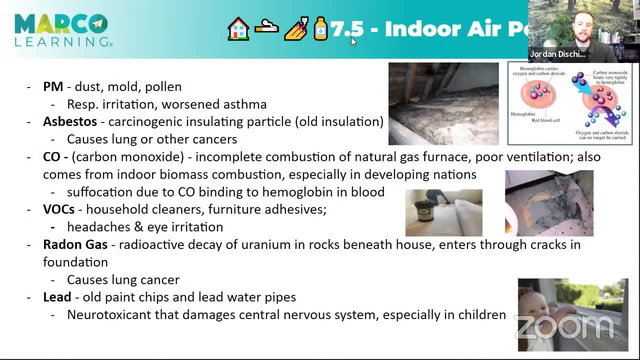 oh nice, smells like a fresh new home. That's actually a volatile organic compound, So that's potentially harmful to you. It can give you a headache. It can irritate eyes, Some of them like formaldehyde, or even carcinogen. 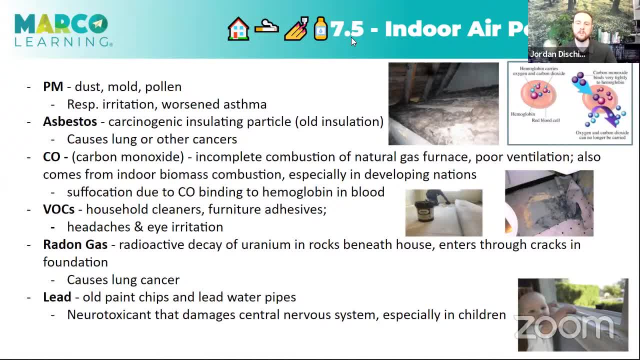 And so volatile organic compounds are another source of indoor air pollution that's in most homes. Then we have radon gas. Radon gas kind of goes into this category with asbestos, where it is a serious retining air pollutant that can trigger the development of cancer, especially lung cancer. 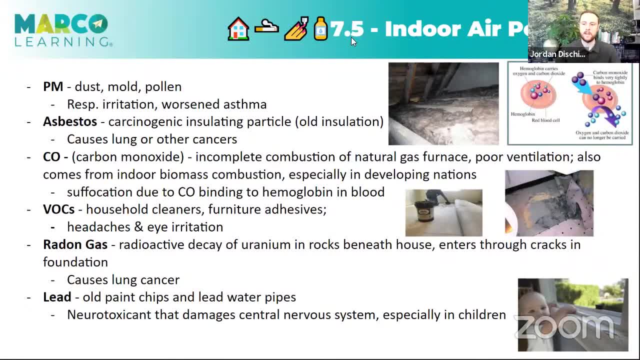 It comes from the radioactive decay of uranium that's found naturally in rocks or in the soil beneath your home. So certain areas of the US are going to be at higher risk of uranium poisoning because of the bedrock that's beneath homes. The way to fix this problem is to seal cracks in your 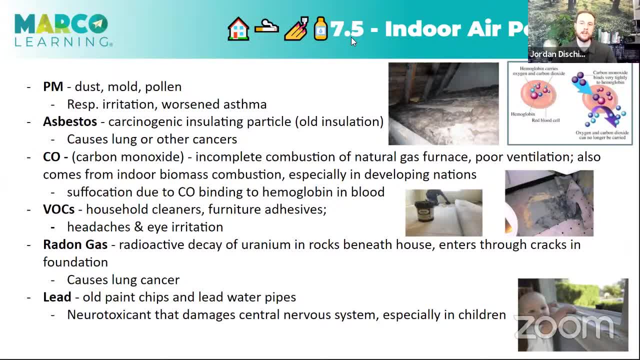 foundation. So if your home has a crack in the foundation, that could allow the radon gas to seep in, And so you can get a radon detector, go around and monitor for levels of radon and then have someone come in, basically put a sealant over those. That's the way to solve this issue And 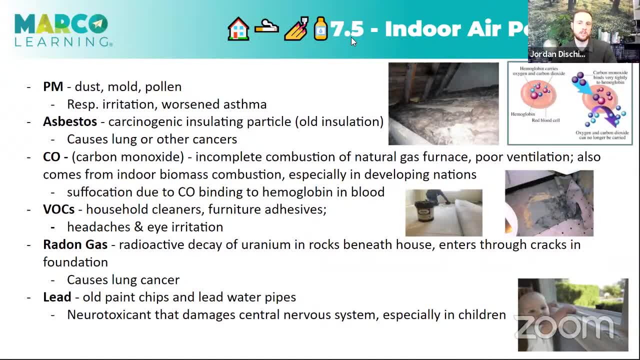 finally, we have lead. As I mentioned earlier, lead can come from old paint chips, So it used to be used in paint. It's not anymore, But many older homes still have this lead paint. It can also come from lead water pipes, So if you 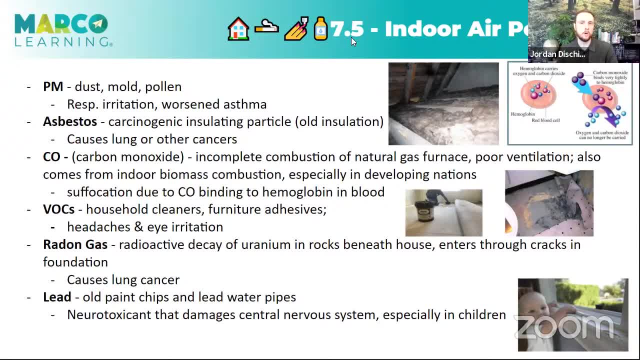 have water pipes that are made of lead. the water can flake that lead off into the water And then when people drink it the lead gets into their bodies. Now, lead is a neurotoxicant, So it's damaging to the central nervous system And we have a picture here of a little baby putting 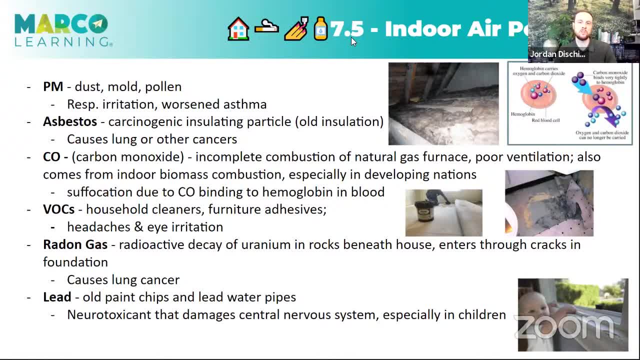 their hands on the windowsill, because it's especially toxic to children. Their immune systems are not fully developed, Their nervous system is still developing, And so the changes and damages that can occur as a result of lead poisoning in infants and small children are especially problematic. So that's something. 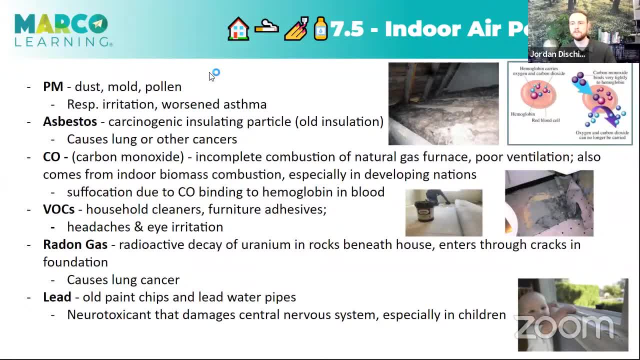 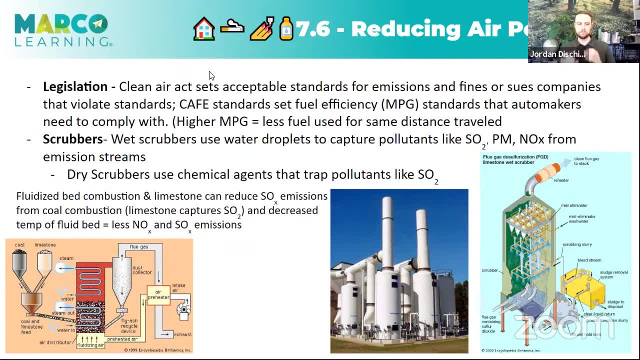 to understand about lead as an indoor air pollutant. All right, So 7.6.. We're going to go through here Now a couple of ways to reduce air pollutants. Now the first one. I really want to call your attention to legislation. One of the number one mistakes that I see APE students make is saying: 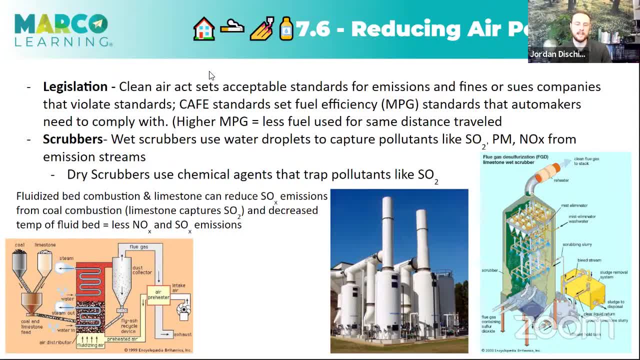 that the government should do things that it can't. Examples would include it should just increase the price of lead, or it should just ban lead, or it should just not let people build new coal-fired power plants. So you have to be careful and really talk about things that the government can actually do, And 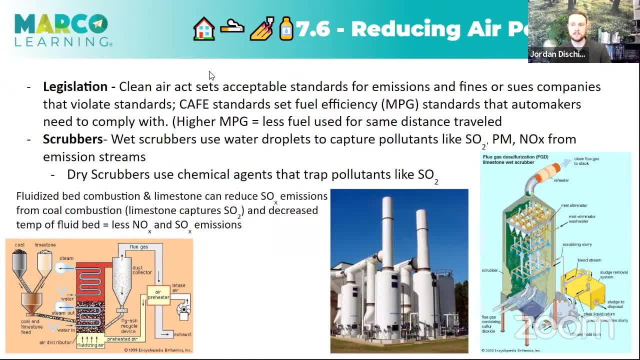 so the Clean Air Act is a great example. The Clean Air Act already exists, And what the Clean Air Act does is that it sets acceptable levels of pollutants for the six criteria- pollutants that were on the first slide from this video on the 7.1, you know air pollutants. beginning, And so what can happen here is the EPA can sue companies or can find them. If they're able to review the air pollutants and think of them for air pollution, They're not going to have any higher levels of pollutants and they're going to have quite a lot of pollutants. 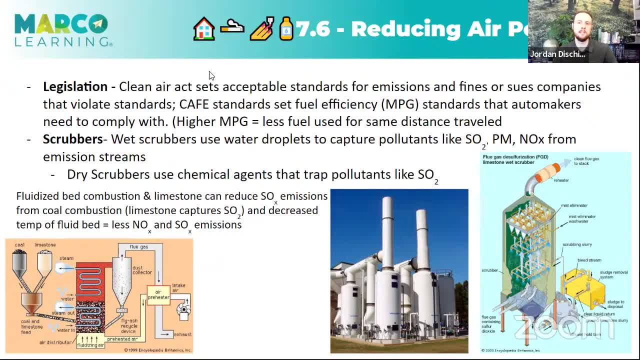 If you look at the results, the EPA is going to be able to have a leading pool for air pollutants in the world, And so next, There's a lot of evidence that we don't get that data, And so what can happen here is the EPA can sue companies or can fine them if they are. 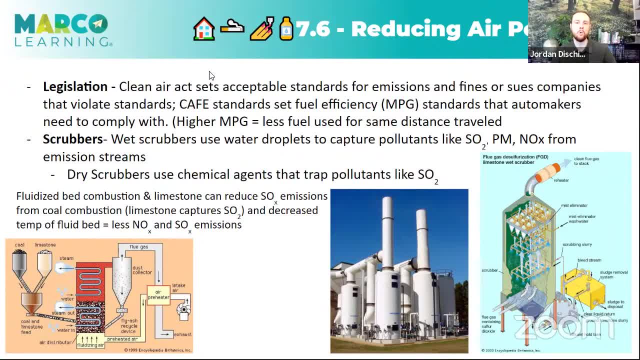 violating those standards. So if they're releasing more, let's just say, sulfur dioxide, SO2, from a coal-fired power plant, if this coal-fired power plant releases more SO2 than the level that the EPA says is acceptable under the Clean Air Act, that power plant could be given a fine. 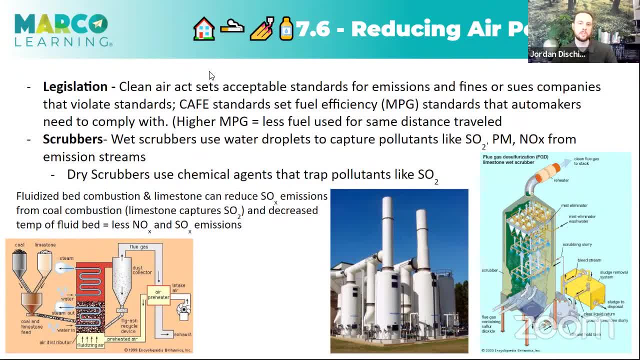 Now that can correct the behavior, That can bring down the emission of SO2 from the power plant. But just saying that the EPA or the government should ban coal is probably not realistic Now. maybe someday we'll get there, but for the most part on an FRQ you should stay away. 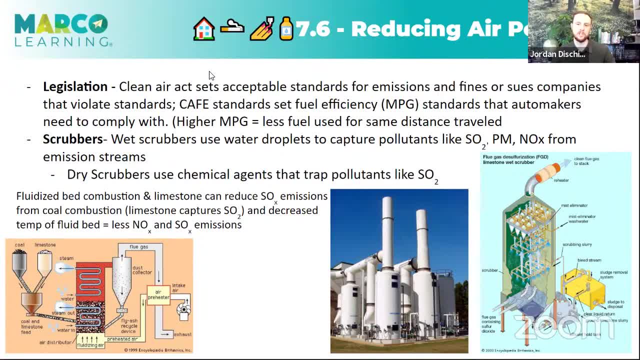 from banning things and stick to legislation that already exists. Then we have the CAFE standards. The CAFE standards set fuel efficiency standards. That means MPG standards, miles per gallon for automobile makers. Now, if the CAFE standards are raised, that means that the average fuel economy of vehicles 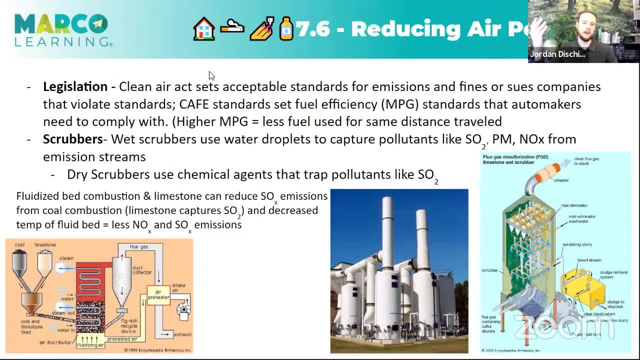 produced by a company like GM would have to come up to that level. So 35 miles per gallon might be an average that's required someday. If that's the average, what that means is trucks that average 20 would need to be offset by a car that's averaging 45 or 50, I should say, to balance it out. 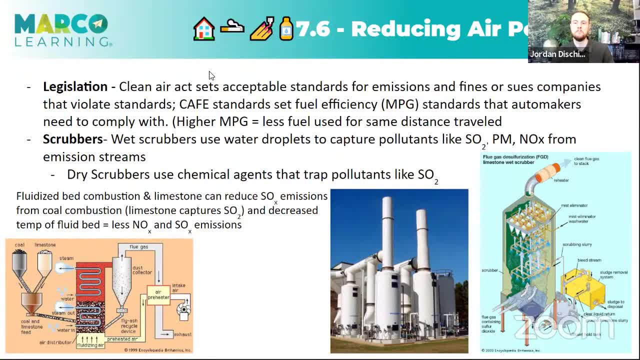 And so what it does is? it means that cars, if they don't get more miles traveled with less fuel or less fuel used for the same distance, travel. so that's how you're going to actually reduce air pollutants, because the vehicles are emitting fewer air pollutants per mile. 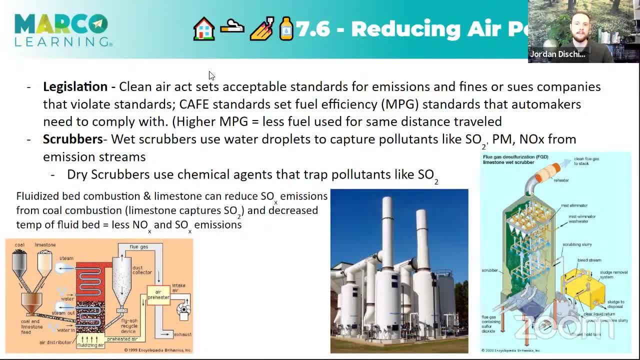 And so really important things to keep in mind there. Clean Air Act and CAFE standards- great ways that the government can limit air pollutants. Now, if we look at smaller solutions, these would be solutions that small emitters themselves could employ. So one specific factory could install these next solutions we'll talk about, or one specific 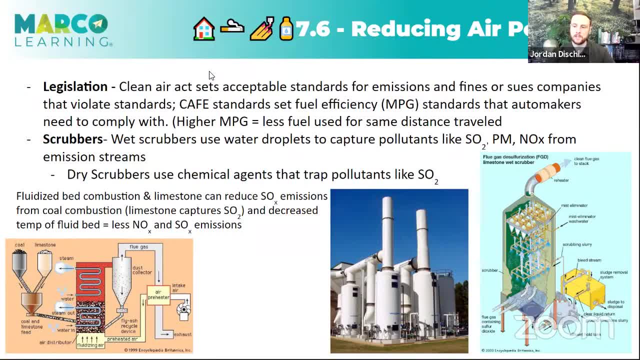 power plant could use these. You have scrubbers, and those include both wet and dry scrubbers. A wet scrubber, as we can see here on the right side of the screen, would basically have all of the emissions or all of the gas fumes from a furnace or from some sort of 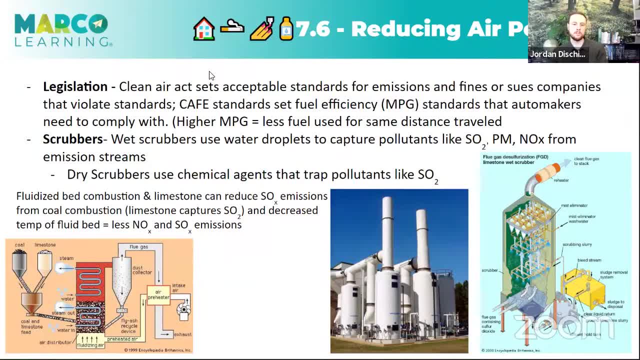 burning, combustion process or manufacturing process, passing through this big column. Then you have mist droplets that are kind of falling, And those water droplets are catching pollutants in the air, pulling them down to the bottom into a sludge tank so that they don't exit the top with the emissions. 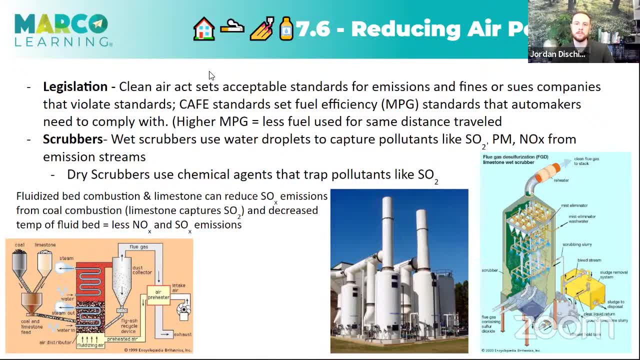 And so what that means is what's coming out of this power plant is much cleaner because a lot of those pollutants are trapped. Then you have a dry scrubber, which is in this middle diagram, here, these white columns. Those are just going to have chemical agents in them that track pollutants and convert. 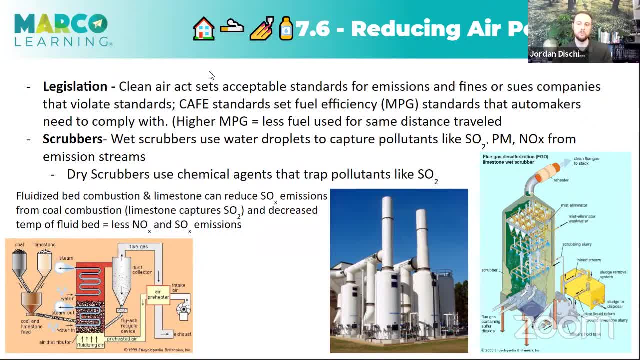 them to a different chemical compound that's solid and stays in the tank. Great example would be sulfur dioxide. And so similar idea, but instead of trapping it with water, they're trapping it with some sort of chemical agent. And then, finally, we have fluidized bed combustion. 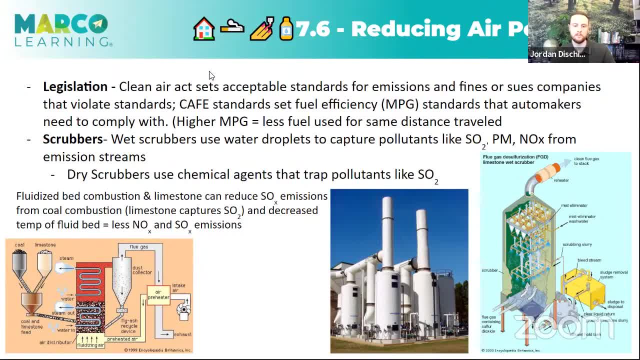 Fluidized bed combustion is where you bubble air into your crushed up coal that you're burning, And you can even add limestone to the mix as well, because limestone will capture SO2 and reduce the amount of SO2 that's being emitted. Also, because fluidized bed combustion allows you to burn your coal at a low temperature. 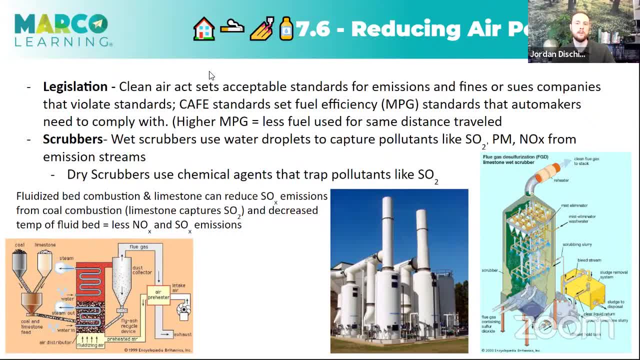 you can also burn your coal at a low temperature temperature. Lower temperatures lead to lower NOx, NOx or NO2 emissions and lower SO2 emissions, And so two methods that can be actually combined to really reduce the SO2 emissions. Again, the limestone will form a chemical reaction that will trap the SO2 in the limestone. 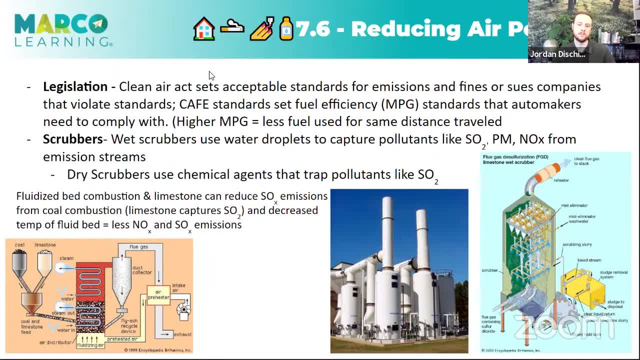 and not allow it to be released in the emissions from the facility. And then fluidized bed combustion lowers the burn temperature because it pumps all this oxygen in. that makes the fire more efficient. And when you lower the burn temperature you lower the amount of NOx and SOx. 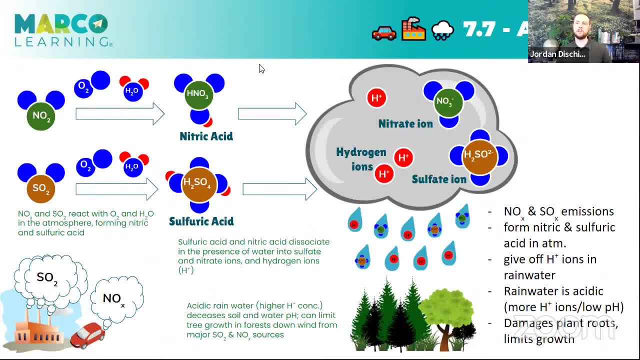 emitted. The final topic that we'll talk about here in 7.7 or in unit seven is 7.7, and that's acid rain. Acid rain is another great example of a chemical equation or a chemical concept that you should understand. So we have SO2 and NOx being released here by a coal-fired. 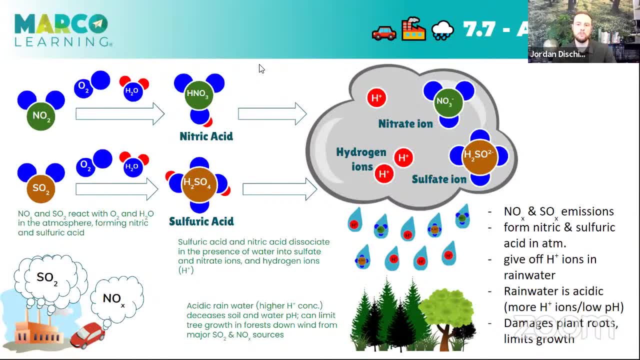 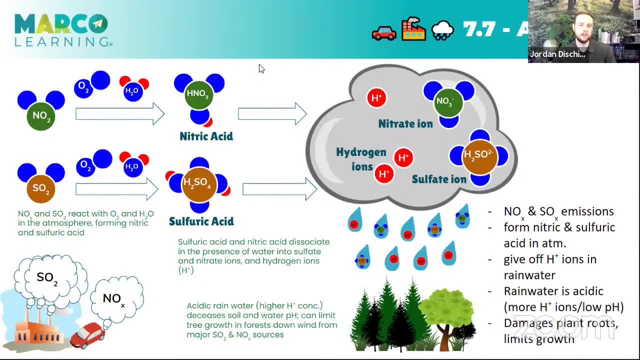 rain formation. One thing I want to make clear, though, is that for smog- for photochemical smog- we're only talking about NO2.. So don't get those mixed up. Don't think that SO2 also contributes to photochemical smog, because it contributes to acid rain. Make sure to keep those separate. 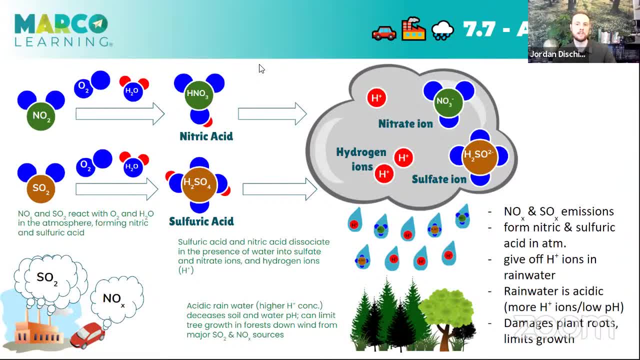 What happens, though, is the NO2 and the SO2 combine with oxygen and water in the atmosphere. That forms nitric acid and sulfuric acid. You don't have to memorize the formulas. If you know them, it helps, because you can remember that we're just adding more hydrogen and more oxygen. 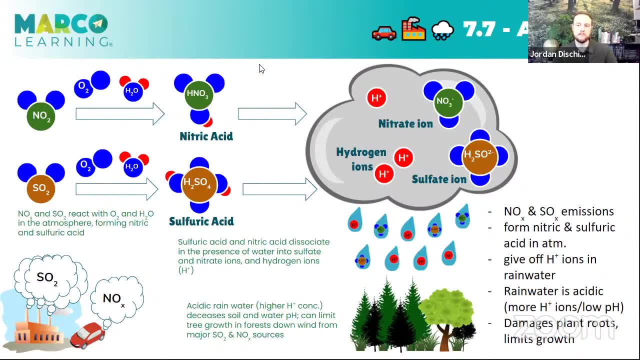 to both of these compounds And that's how we get nitric acid and sulfuric acid. Those would be secondary air pollutants, because they form from primary air pollutants undergoing a transformation. Then what happens is in water these acids dissociate. Dissociation is when you 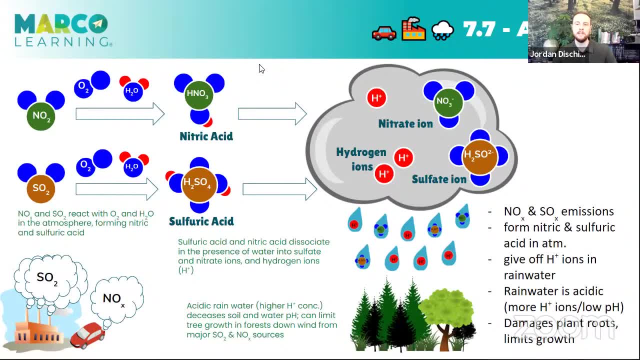 form two ions, one positively charged, one negatively charged. In this case, the positively charged ion is a hydronium ion or H plus ion. Then what you have is the nitrate ion, and that's NO3 minus, and the sulfate ion, H2SO2 minus. 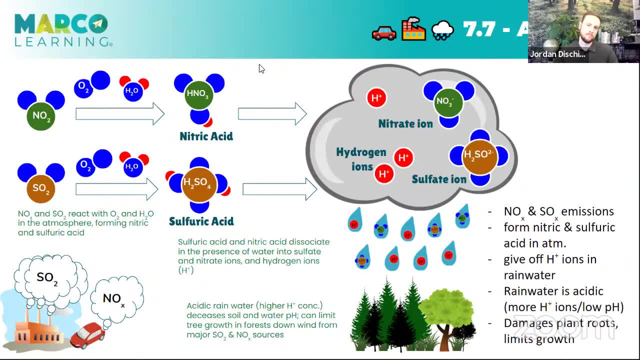 And so I should say H2SO minus two. But when you form these ions, what's going on here is the H plus ions are getting into the rainwater, And when you increase H plus ions, that lowers the pH. That's what acidity really is. It's a measure of H plus ions. 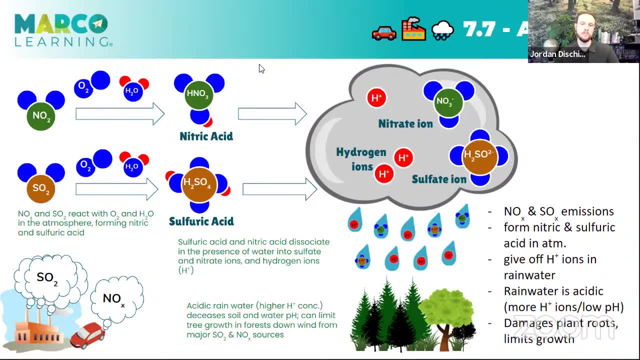 Another thing you can do to really take your FRQ writing to the next level, to really take your understanding of H to the next level, is understand what does pH measure, What does acidity actually mean, And what acidity actually means is higher H plus ion concentration. 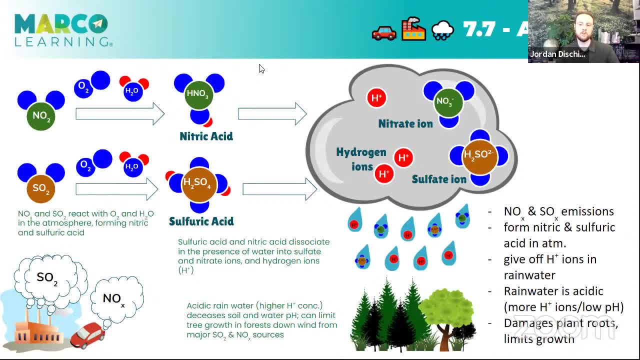 The reason I say that's helpful to understand is if you know your soil chemistry, you know then that H plus ions displace other positively charged macronutrients, things like calcium or magnesium, which have positive charges. So those H plus ions, that acidic rainwater when it falls down to an ecosystem. 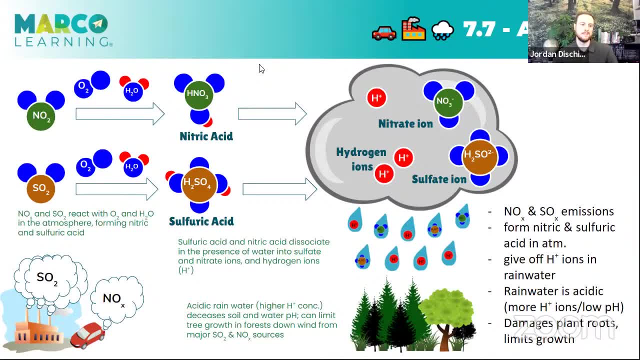 it can damage plants' roots, It can make them more susceptible to diseases, It can leach nutrients that they need out of the soil and they are no longer able to grow and repair their tissues and make new leaves and fruit and all of the other. 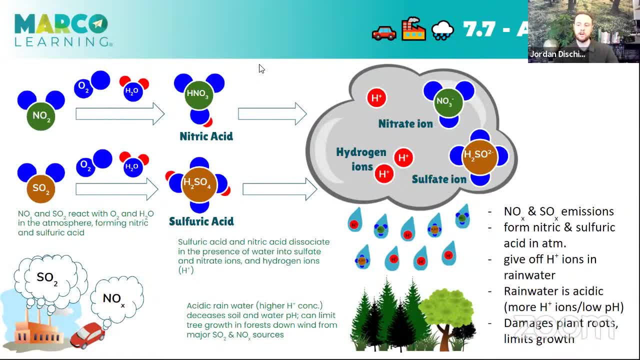 things that plants need to be able to do. So acidic rainwater is really problematic for plants especially, And many amphibians as well can suffer, you know, sublethal effects Like infertility or physiological stress because of all of those H plus ions in the acidic rainwater. 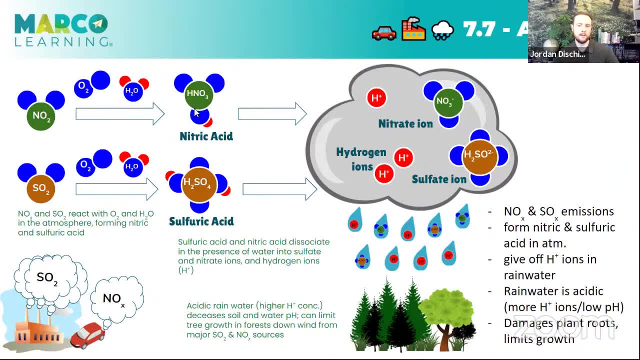 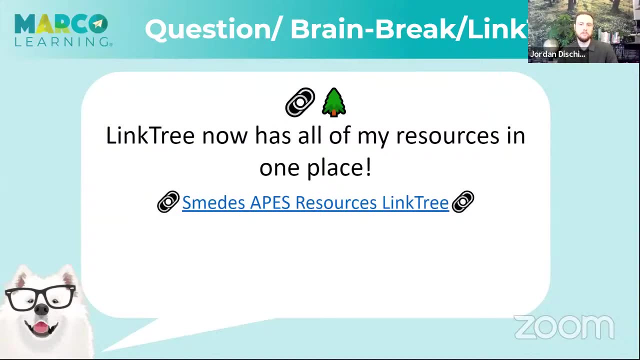 Hey Han Yan, thanks for commenting Acid rain. the diagram's cool, but the concept itself not so cool, especially if you're at three. So thanks for the comment, though What I want to do is pause here for a second, because that was a lot. We went very fast and 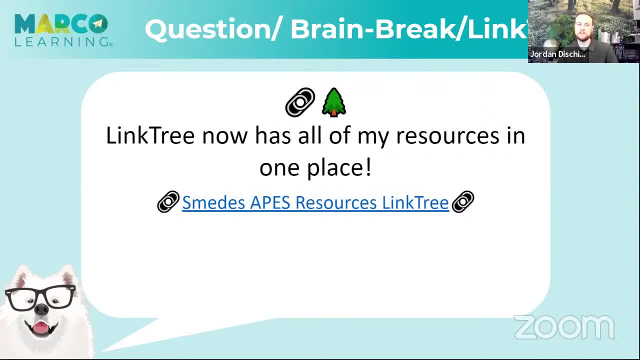 we have just a couple minutes left And we're going to wrap things up at 3.45, so that's only four minutes from now. We're going to wrap things up at 3.45,, so that's only four minutes from now. 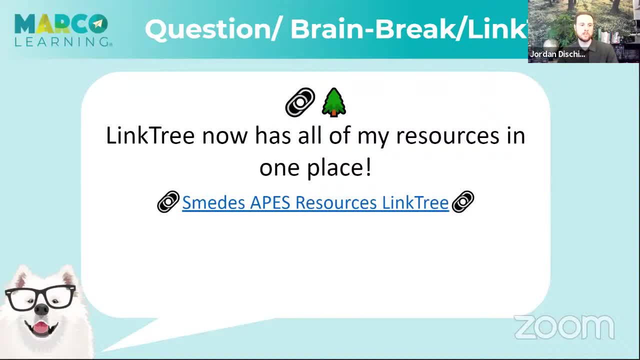 So I want you guys to take a second to think about what we just covered, See if you have any questions and ask those in the comments while we're still rolling here, And then, as you do that, I'll take a quick break, grab a drink and then I'll pop the Linktree into the comments. one more. 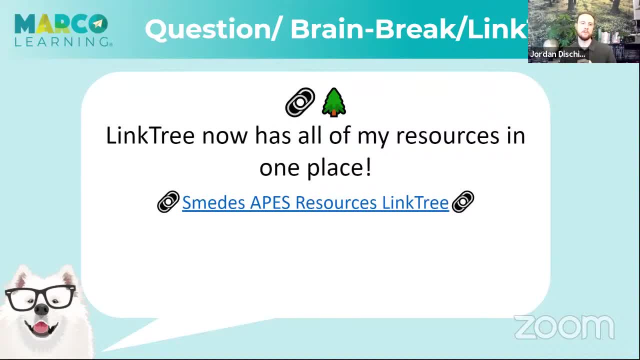 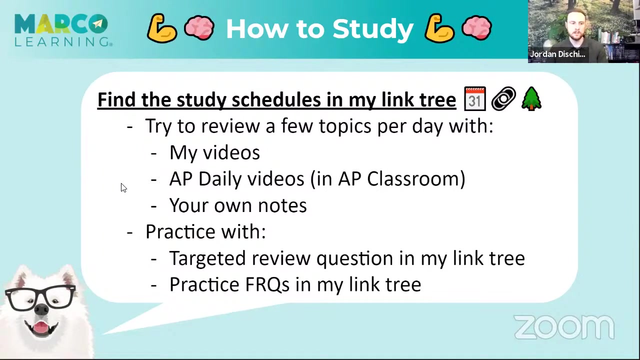 time, because that is a super, super helpful resource And I would love for you to check that out right now, Thank you. So, if you haven't already, go ahead and copy and paste that link from the comments into your browser and check out all of the resources that are on this Linktree, Some resources that I really 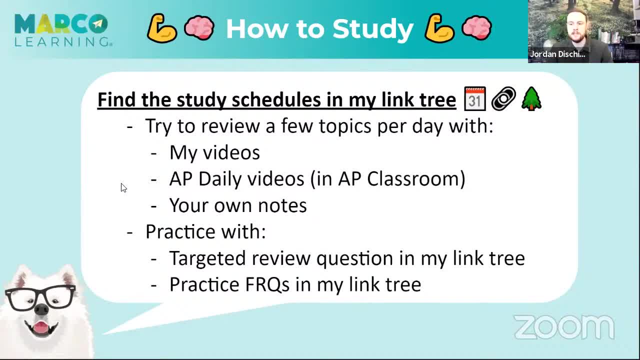 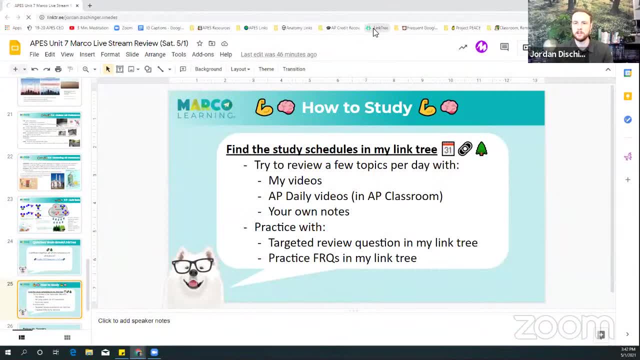 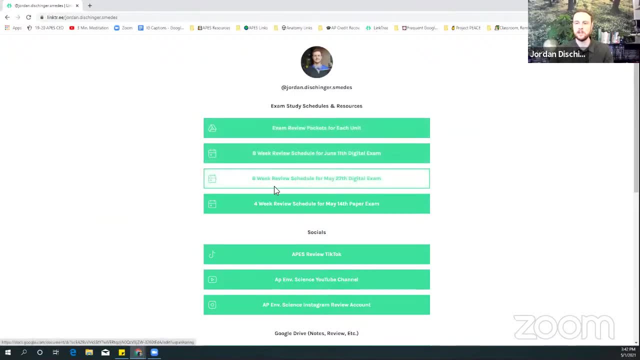 recommend using here would be the daily review schedule, And so I want to actually share this on my screen right now. So I'm going to click on my Linktree here so that you can see what I'm talking about, because this is a super helpful way to study and not get super overwhelmed. 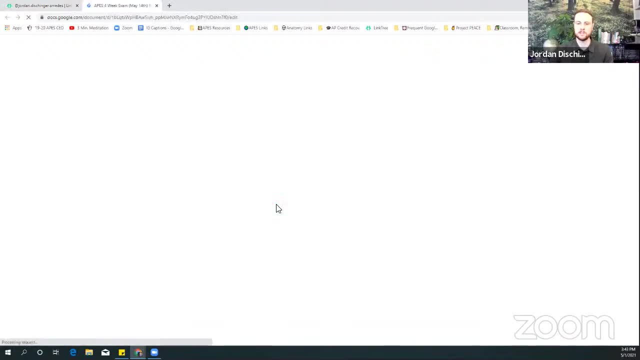 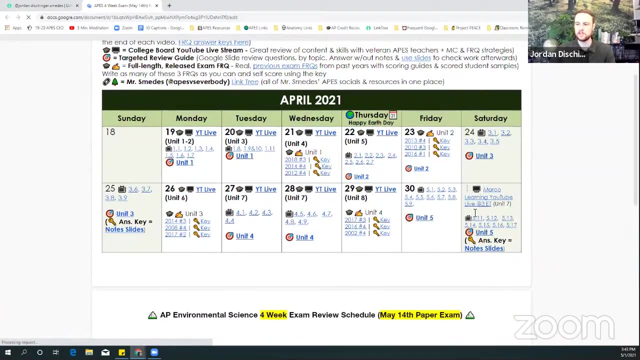 So, depending on when you're taking the exam, like if you're taking the May 14th paper exam- this is a schedule that I put out a couple weeks ago that would help you walk through things. So you can see, today is the first, So I recommend that you're up through about unit five in your 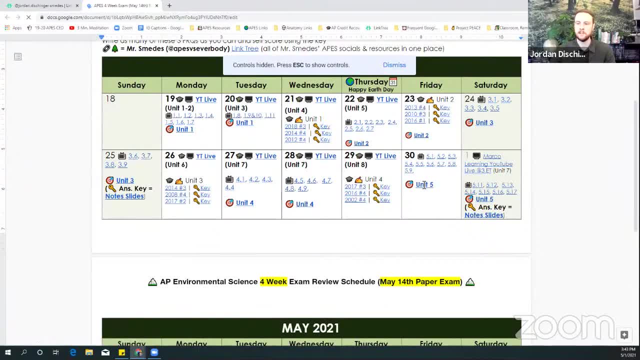 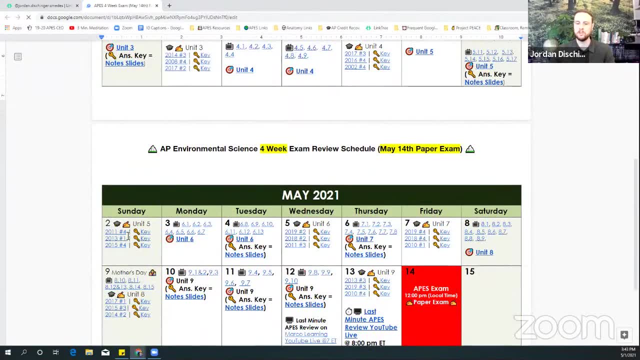 exam review. But don't panic. if you're not in unit five, You can definitely still do some catch-up. but you do need to know that your exam would be coming up on the 14th year, And so you could use these mini FRQs and keys. released FRQs and keys. And then these are all links to my 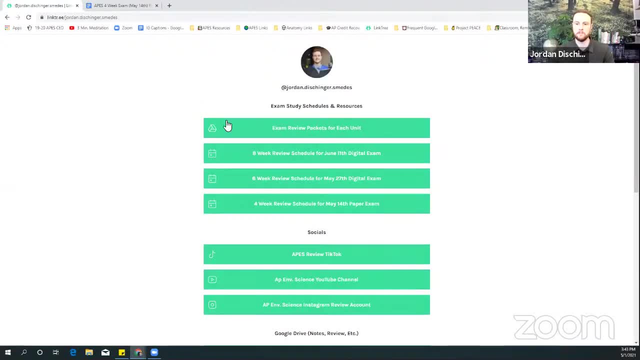 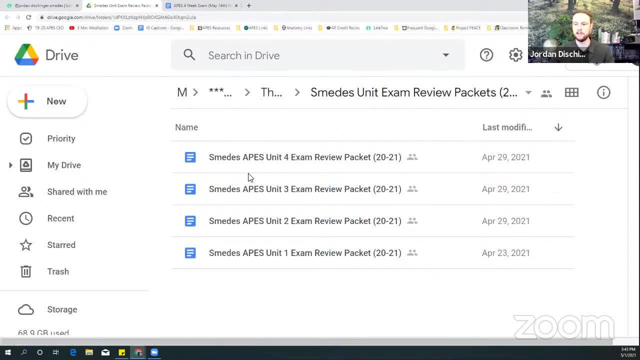 topic videos that I recommend you watch. Another great way to study, though, is to go to these exam review packets for each unit, And right now, I just have through unit four, but I'll be plugging in five and nine later, And what you can do is open this up, and I have 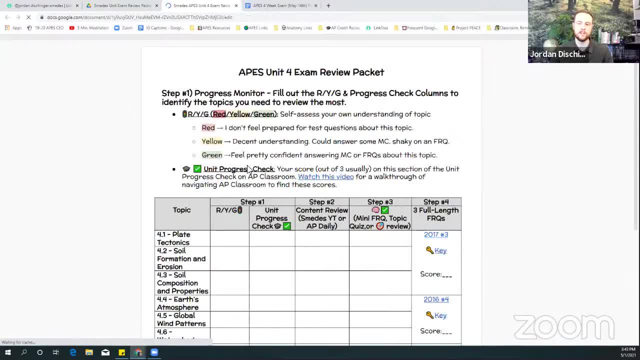 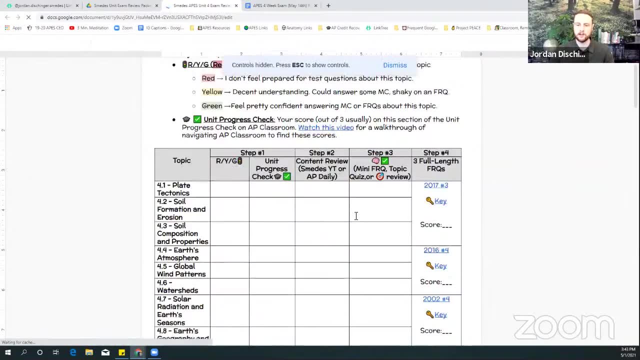 a TikTok that walks you through exactly how to use this. So if you don't already go, if you don't already follow the TikTok, go over there and check that out. But what you want to do is go to the top of the page and ask yourself: which of these topics do I need to study the most? 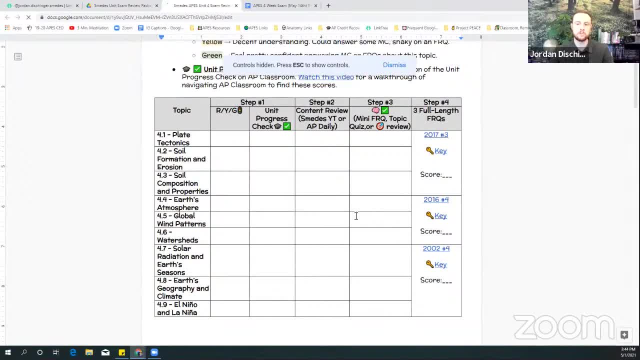 Especially if your exam is in under two weeks, on May 14th. you need to do some targeted study. You can't cover all 99 course topics in two weeks. That's just too short a time. But what you can do is go through each unit and you could use your unit progress checks. I'm in a video on my YouTube. 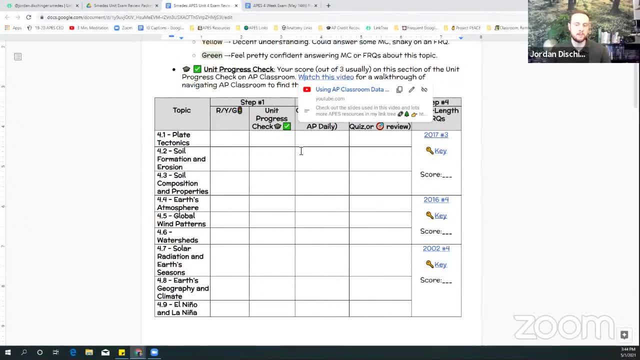 channel where you can go see how to do that And then you can study like your three weakest topics in unit four instead of everything. So that's what I recommend. I hope that makes things seem a little less overwhelming and seem a little more doable. 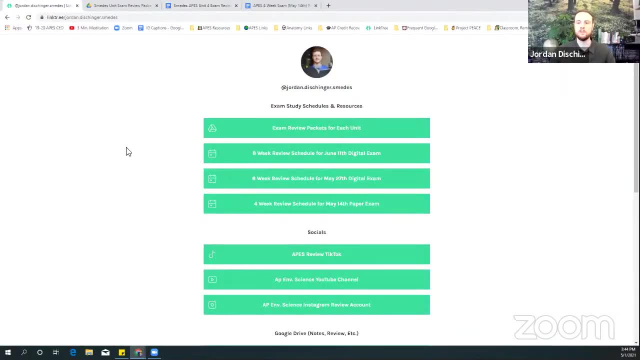 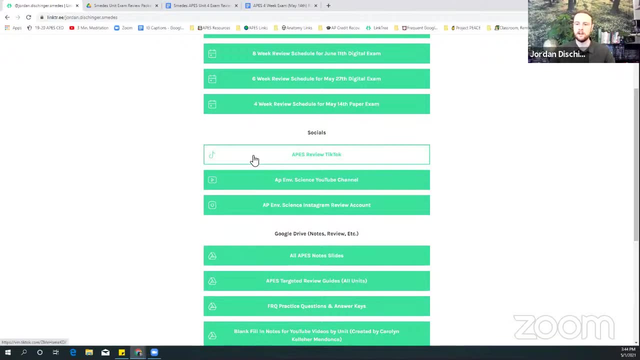 And again, just to point out on the link tree here, all the resources you need to study are here. There's a TikTok which will start having more and more kind of daily concept reviews. Right now it just has study tips. The YouTube channel has everything you need. You want to make. 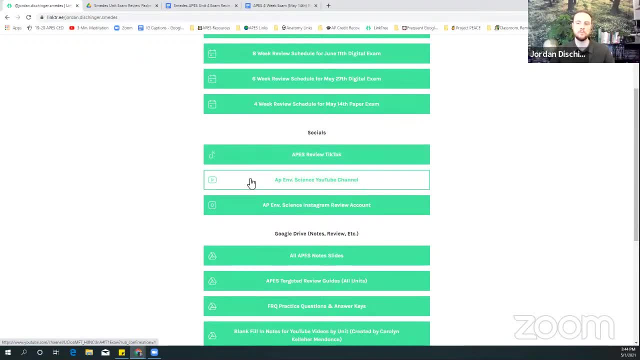 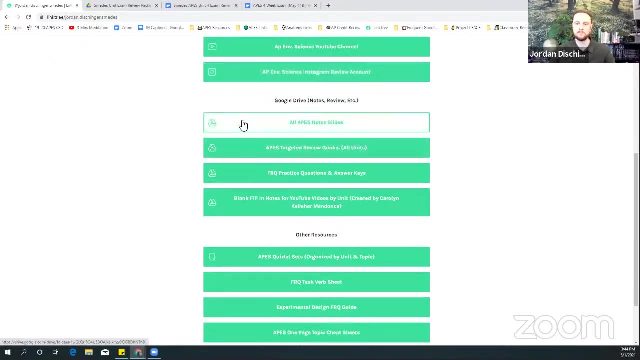 sure to check this out, If you don't already. that's where future videos will be on how to write each of the three FRQs. And then the Instagram account has daily review as well. This is probably the most valuable link in the whole link tree. It's the one that the most people click on. 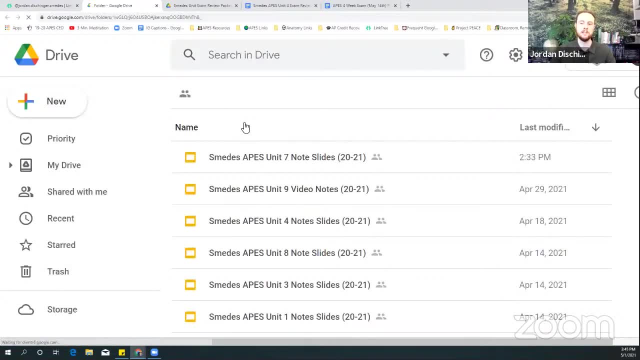 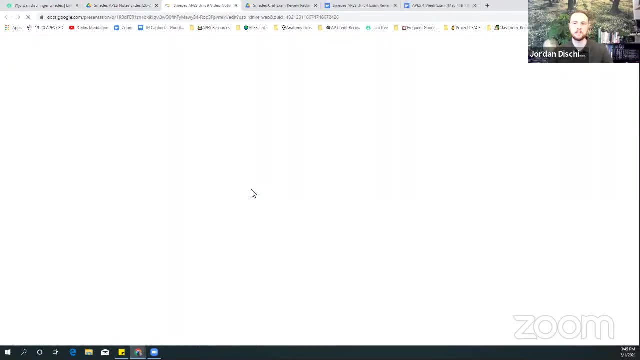 And this is all the APES note slides. So if you want to see everything that's in my videos, exactly what I use to make them, you can click on any of these units and you have access to everything that I use in my videos. And so if you open this up and you go through it, 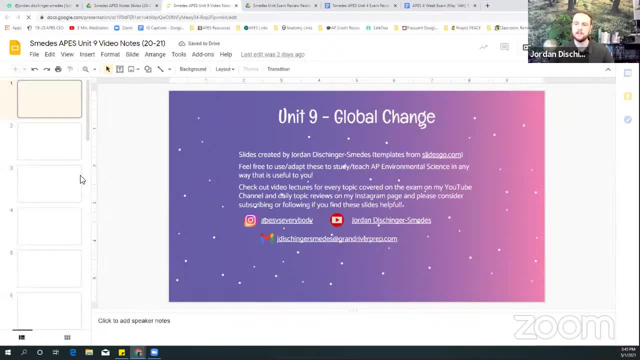 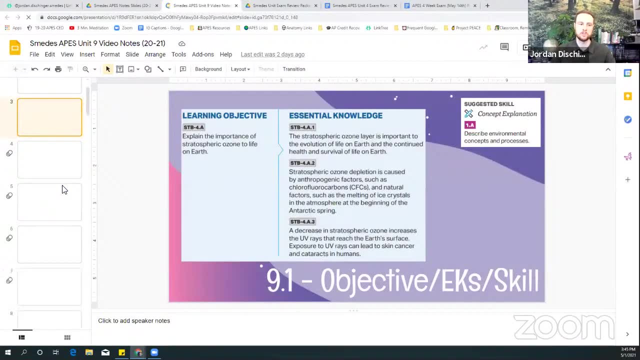 it'll just have for each topic like five to six slides And it really covers the basics of what do you need to know for each topic, So it has objectives. what do you need to know for each topic? what do you need to know for each topic? 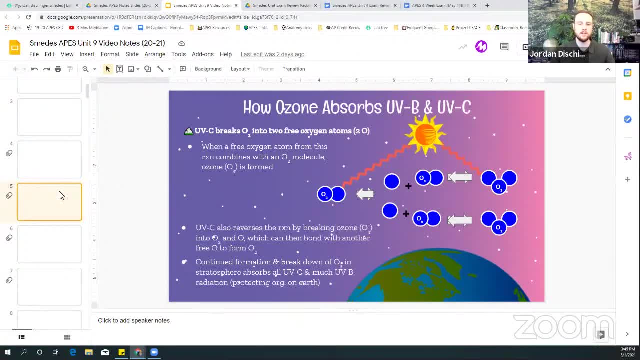 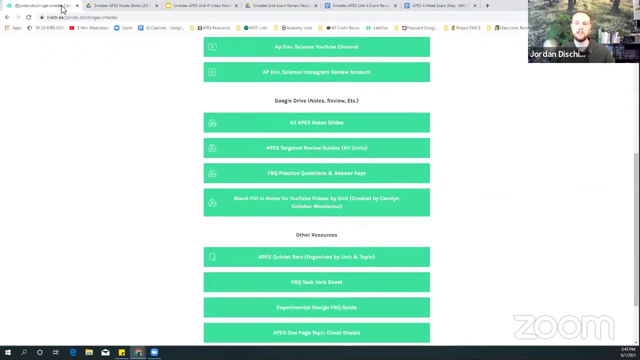 exactly what the college board says you need to know. It has diagrams to break down all of the concepts, And so that is a really, really helpful resource as well. Again, I tried to pull everything into this link tree so that you guys have exactly what you need to study. Lauren has a question. 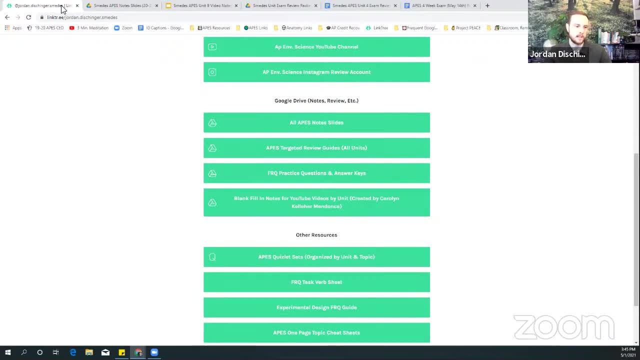 here. How do you recommend we study for the math portion? Will we get enough practice if we just practice FRQs? Here's my advice, Lauren. Don't quote me on this, because it's up to the college board ultimately, but almost all of the courses that you're going to get are going to be in the 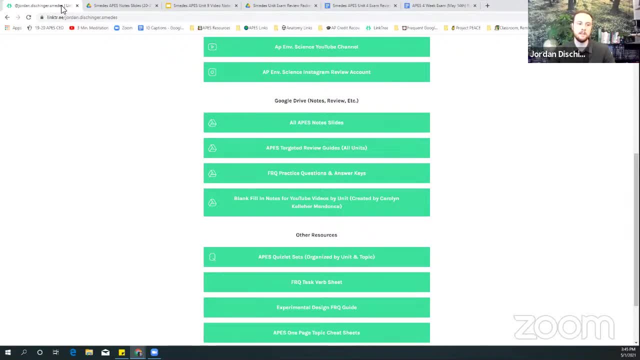 FRQs. Almost all of the FRQs that we have seen of recently are percent change, So really important to know how to do percent change. If you go back to my previous videos of Marco Learning, I go through a couple different percent change calculations, So check out the unit six videos. 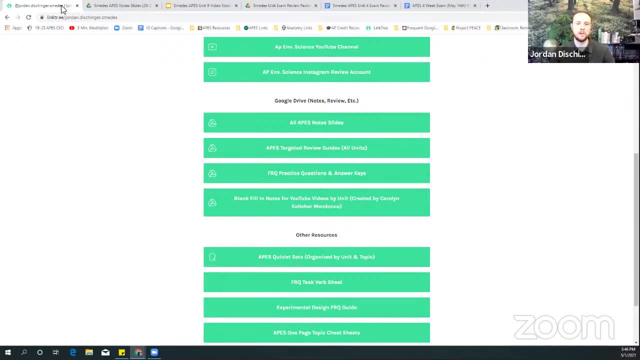 You can go to Marco Learning's channel and you can find those videos. Just search for apes on Marco Learning and you'll see me walking through a few different percent change calculations. Again, the good news is that it looks like the math will probably be percent. 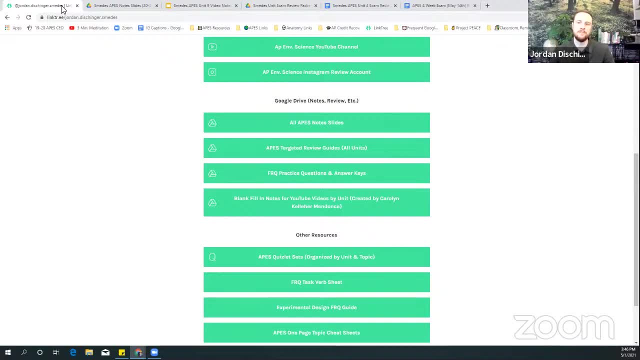 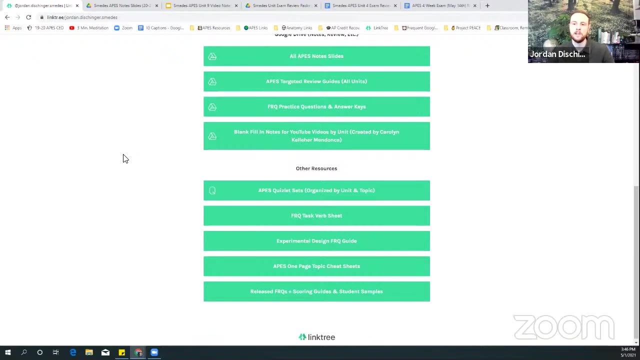 change- Don't quote me on that if you happen to get primary productivity or something else. but percent change is definitely one that continues to appear on FRQs. That would be my advice there. Again, really, really highly recommend that you guys check out the link tree. 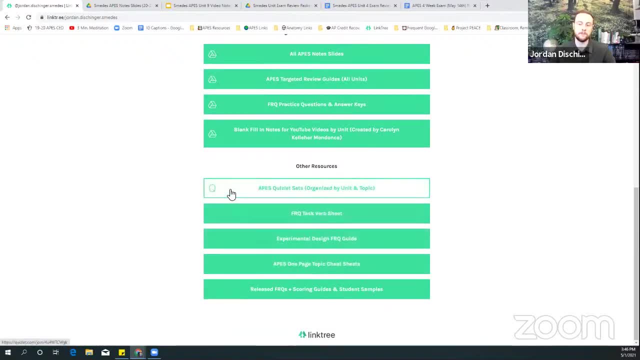 I try to put everything there that you need. A couple other things that are further down the link tree that people don't always make it to would be the Quizlet sets. So these are going to be organized by unit and by topic. Those are going to be helpful things. 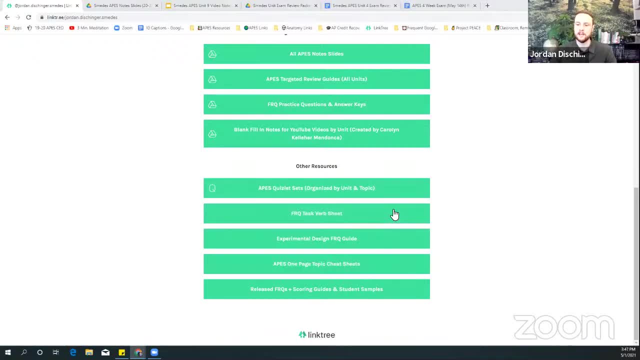 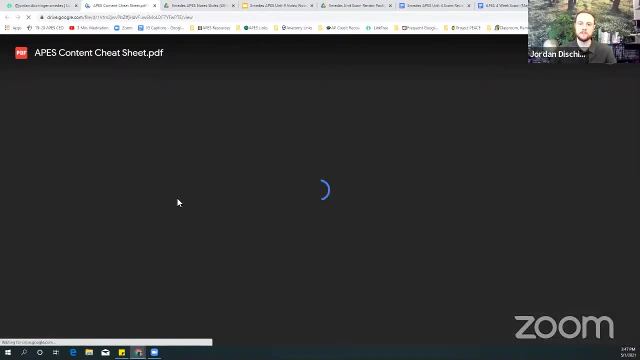 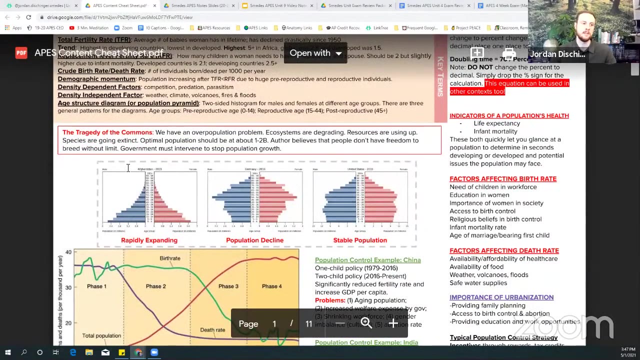 Also the FRQ task verb sheet. And then the other thing, the final resource I would highly recommend checking out would be this one page topic cheat sheet. A teacher on Facebook created this and just has tons and tons of great resources just to remember concepts quickly at a glance.